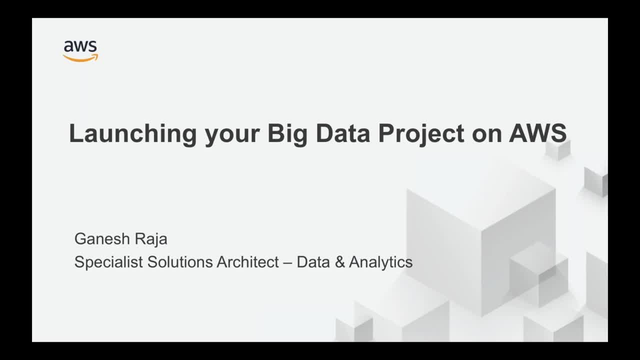 Good morning everyone. Welcome to the launching on your big data project on AWS. I'm Ganesh Raja, a specialist solutions architect based out of the Melbourne office for data and analytics. Today we are going to go over how to build your big data project on AWS and what tools. 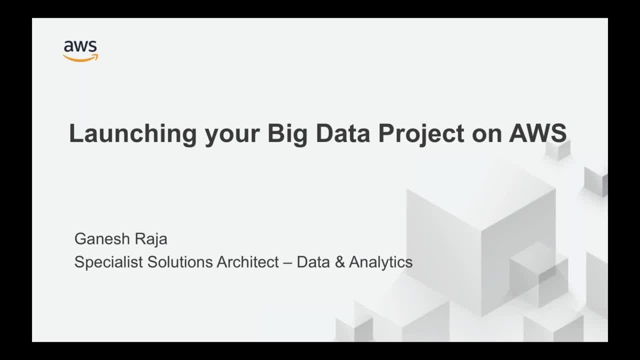 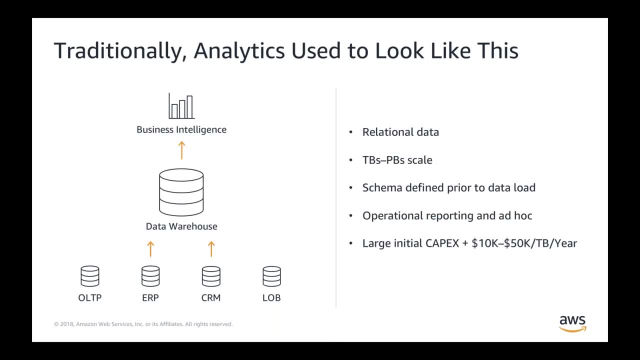 are provided by AWS for you to build your big data project on us. Traditionally, analytics used to look like this: There was business intelligence, There was data warehouse. The data warehouse used to take data from OLTPs of streams, ERPs, CRMs and labs. 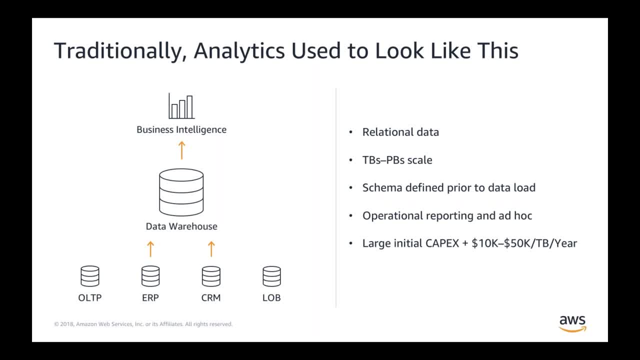 And they used to scale to terabytes of petabytes. There is a large initial capex of 10 to 50k per terabyte per year, And then you have an OPEX cost as well. on top of that, Data lakes extended this. 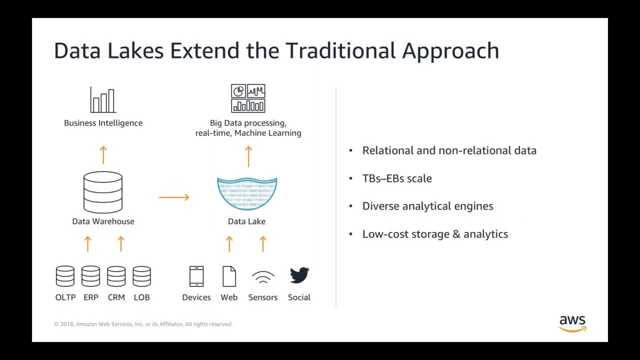 traditional approach. It started looking at both relational and non-relational data. The scale became from petabytes it became exabytes. Diverse analytical engines were able to be run on top of the data lake And it became low cost for storage and analytics. 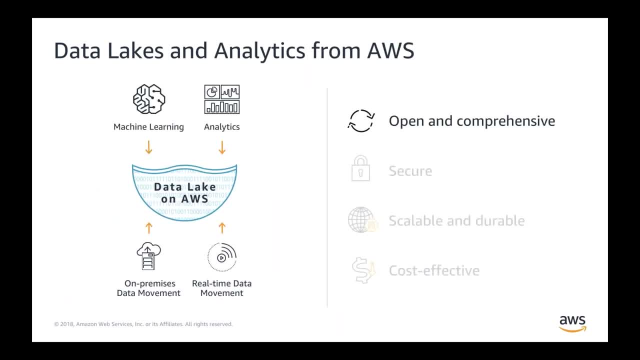 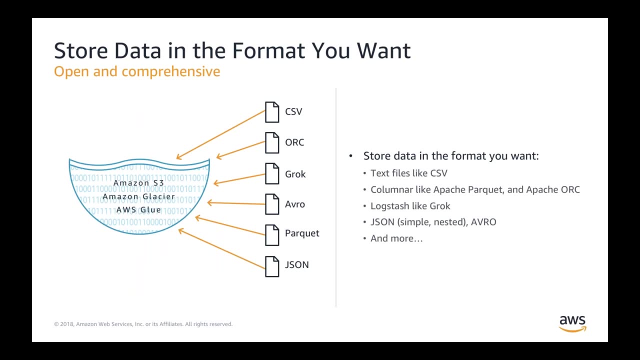 Data lakes and analytics from AWS. we operate on four foundational principles, The first one being open and comprehensive. Customers want the freedom to make the choice where this data is stored and where they want to store the data. Store the data in the format that. 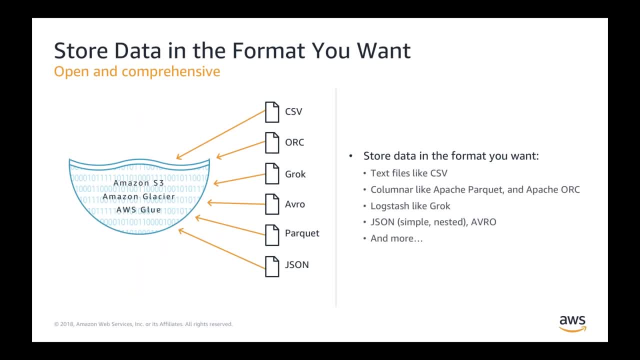 you want Text files, columnar files like Apache Parquet, Apache ORC, Logstash like Gawk, JSON and more. You can store the data in the format that works for you. Apart from that, we also want the data lake to be secure. AWS provides the highest levels of. 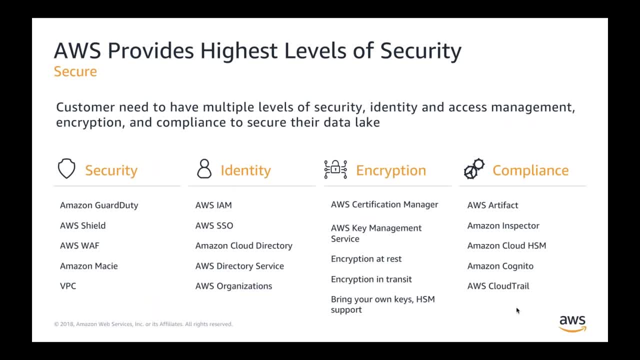 security. It has security for those of you in the Another world and the other world. It has the highest security for those of you in the Other world. It has security for those of you in the Other world. It at various levels. It has encryption and compliance as well. Security is machine learning powered. 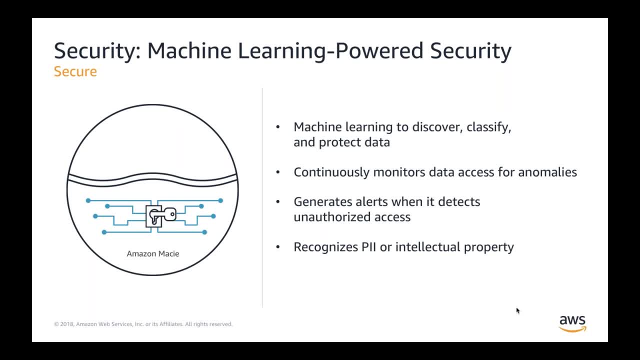 security. Machine learning to discover, classify and protect data. continuously monitor data access for anomalies, generate alerts when it detects unauthorized access. The fully managed service called Amazon Macy continuously monitors data access activity for anomalies and generates detailed alerts when it detects risks of unauthorized access. on inadvertent data leaks: 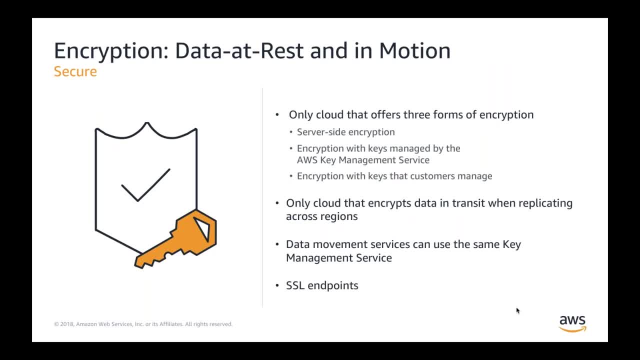 Encryption at data at rest and in motion. We are the only cloud that offers three forms of encryption: Server side encryption. encryption with key managed by the AWS. key management service. encryption with keys that customers manage as well. It is the only storage offering that. 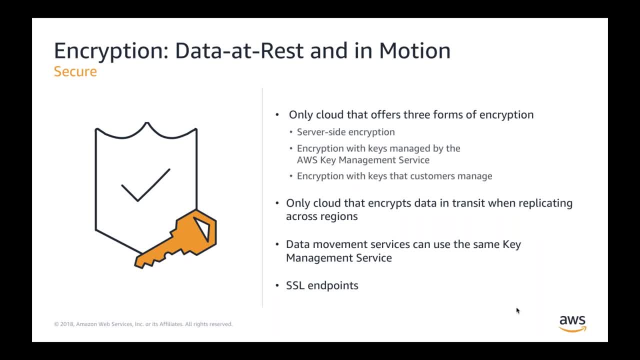 encrypts data entranced concept when replicating across regions and list customers. use separate accounts for source and destination regions to protect against malicious insider deletions. We provide you SSL endpoints for all data coming in or going out, So all of the APIs are over an SSL endpoint. 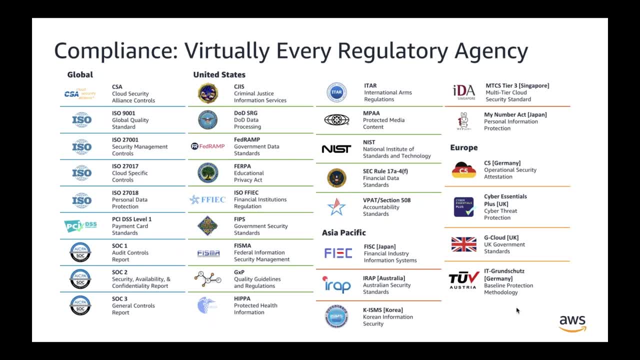 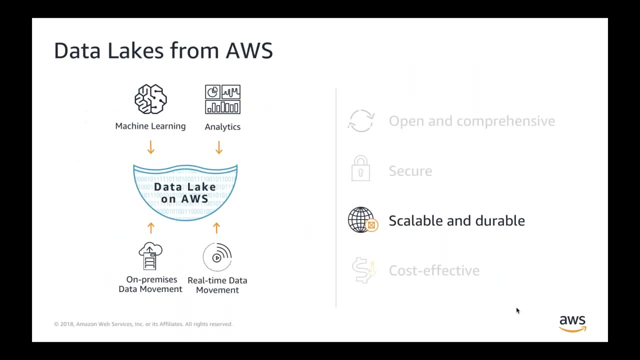 AWS supports security standards and compliance certifications, including PCI DSS, HIPAA, ITEC, FedRAMP, EU Data Protection Directive and FISMA, which can help customers satisfy compliance requirements for virtually every regulatory agency around the globe. The data lake from AWS is also scalable and durable. S3 has trillions of objects and exabytes. 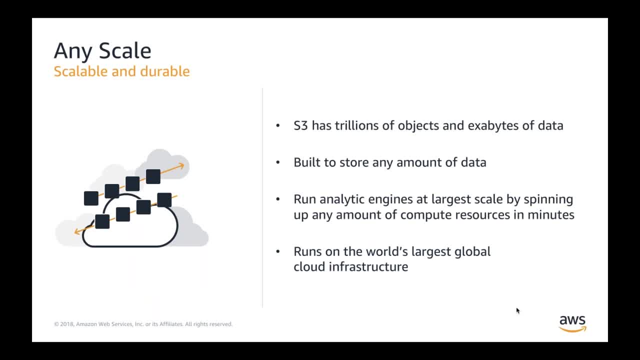 of data. As data volumes grow, customers have traditionally made a choice between purchasing and installing larger, more powerful hardware, or making decisions on what data should be stored and what data should be discarded. Amazon S3 eliminates the need to make this choice because it is built to store and retrieve any amount of data It runs on the world's. 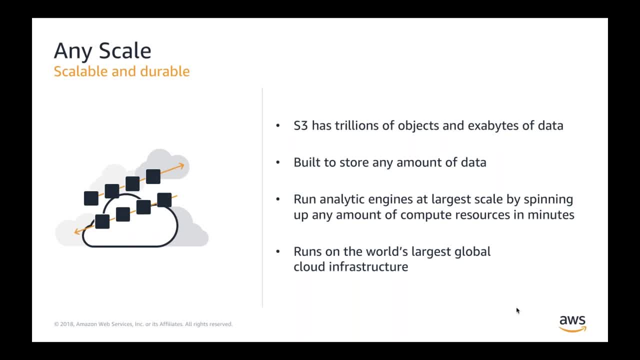 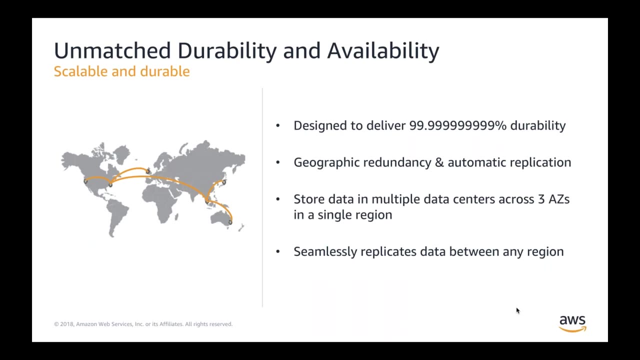 largest global cloud infrastructure and you can run analytical engine on at the largest scale by spinning up any amount of compute resources in minutes. S3 is designed to deliver 11 nines of durability, geographic redundancy and automatic replication. Unique capabilities include storing customer data and independent data centers across three availability zone. 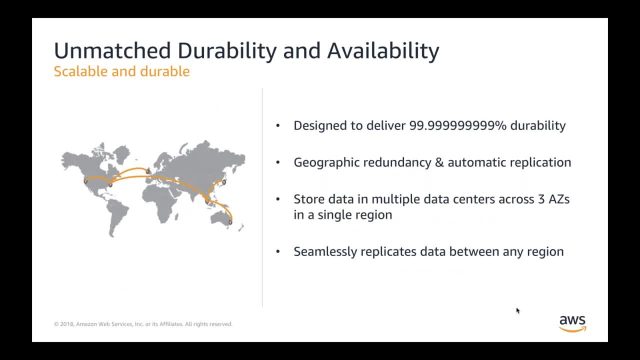 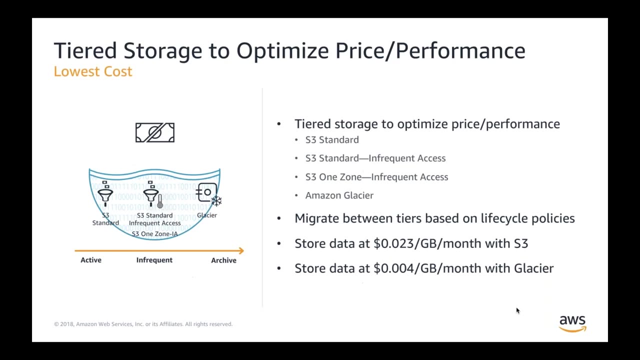 within a single AWS region and automatically replicating data between any region, regardless of storage class. The data lake from AWS also has a lowest cost of ownership. It provides you tiered storage and to optimize price and performance. Storing large and growing volumes of diverse data can be costly, with a lot of infrastructure to acquire Data lakes. 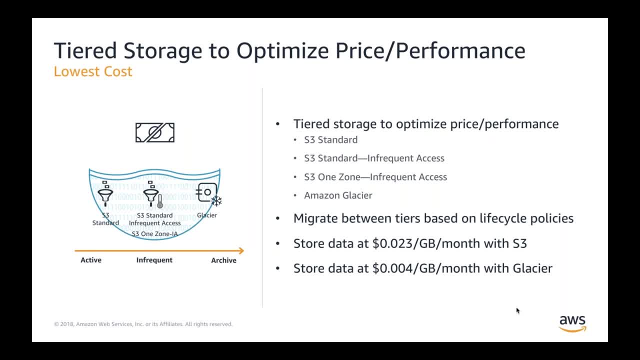 built on AWS are the most cost-effective. data that is infrequently used can be moved to Amazon Glacier, which provides long-term backup and archive at very low cost. Amazon S3 management capabilities can analyze object access patterns to move infrequently used data to Glacier on demand or automatically with lifecycle policies. 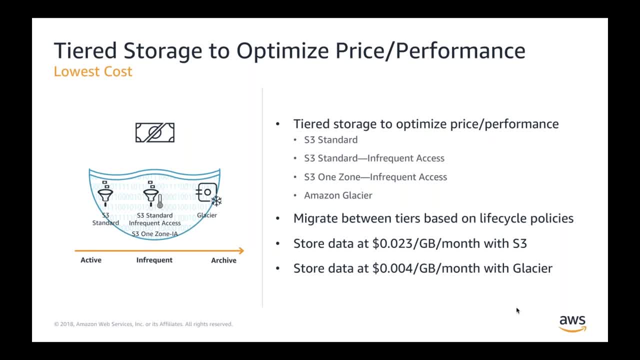 Amazon Glacier is built on the same highly reliable infrastructure as Amazon S3.. Running analytics on the data lakes can be expensive and time-consuming because large amounts of data are stored in objects and each query returns the entire object regardless of what is needed. Amazon S3 Select uniquely retrieves only the subset of data within an object. 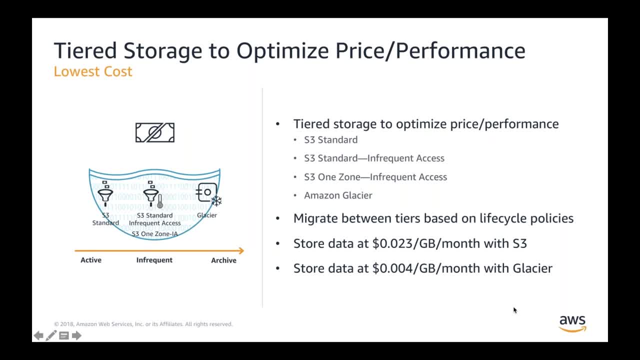 leading to much faster queries- up to 400% faster and at a dramatically lower cost For customers that want to query archived data. Glacier provides Glacier Select a similar capability to S3 Select. The storage costs are as mentioned here. in US dollars is 0.023 cents per GB per. 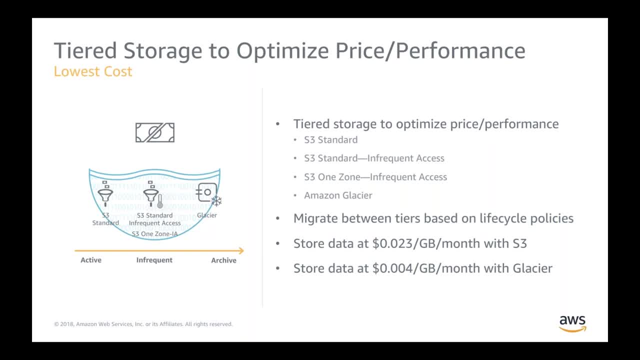 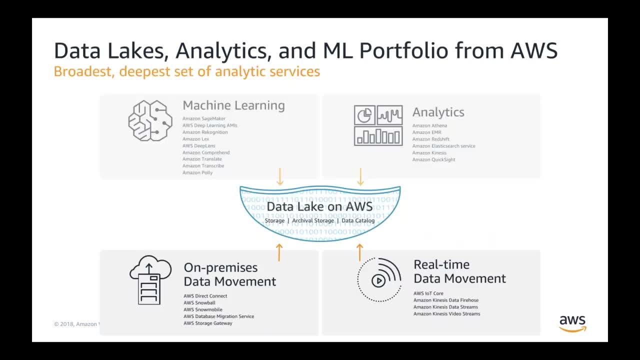 month with S3, and 0.004 cents per GB per month with S3, and 0.004 cents per GB per month with Glacier. The data lake on AWS gives you the broadest and deepest set of analytics services. Let us look at how we can hydrate this data lake on AWS. 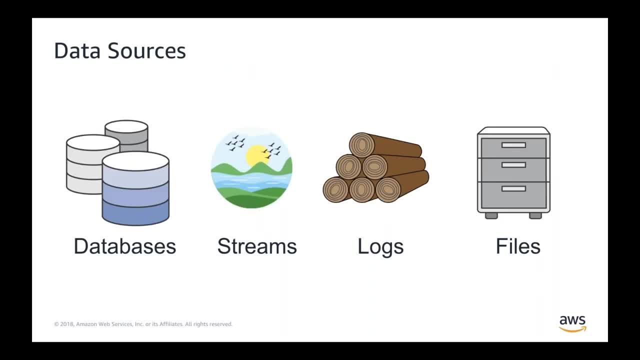 Hydrating the data lake on AWS comes from multiple data sources. There are a lot of places that data can come from. Predominantly, these fall into one of four categories — files, logs, streams and databases. files can come from self-hosted file systems or via third-party data feeds via ftp or api streams. 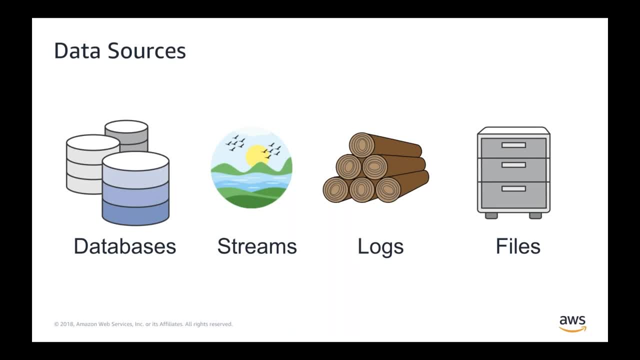 are open-ended sequences of time series data that has clickstream data from a website or iot device, usually published into an api that we host. logs get generated by applications services operating systems. the data lake is a great place to store all of these for centralized analysis. 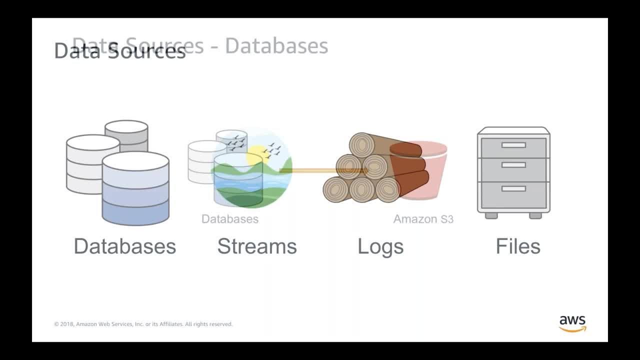 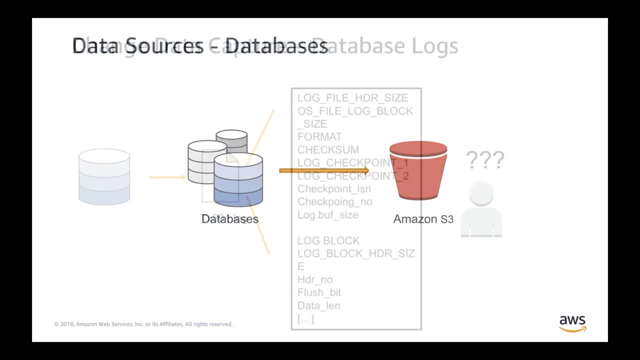 and, of course, your databases comes in. all sorts of flavors these days, both relational and drawn traditional. let us look at how aws services can help you move your database to amazon. s3. databases have a way to capture changes that are being made in the database in into a time-stamped series of files, while it may be known under different. 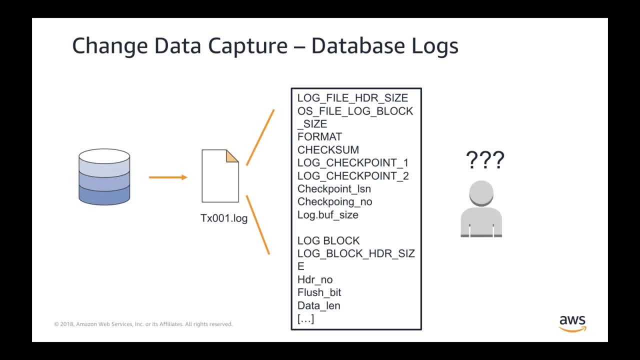 names, but it can be used to capture changes that are being made in the database into a time-stamped series of files, while it may be known under different names depending on the vendor. the transaction log is where the engine writes all ddl activity, making it a perfect way to asynchronously process record changes without impacting the performance. 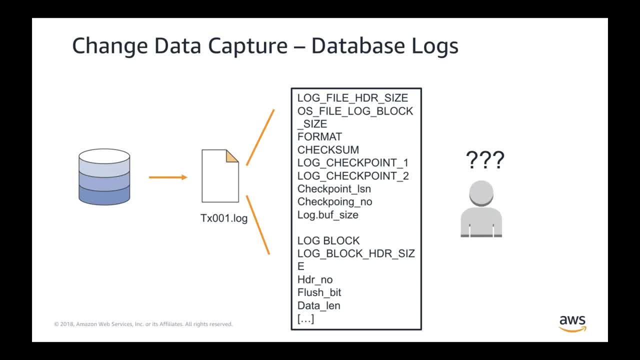 of the engine itself. it also guarantees that no record change will ever be missed, with the ability to replay a change should the initial attempt fail. the problem is transaction logs are very difficult to decipher, often undocumented and considered proprietary to the vendor. accurately reading and consuming a transaction log. 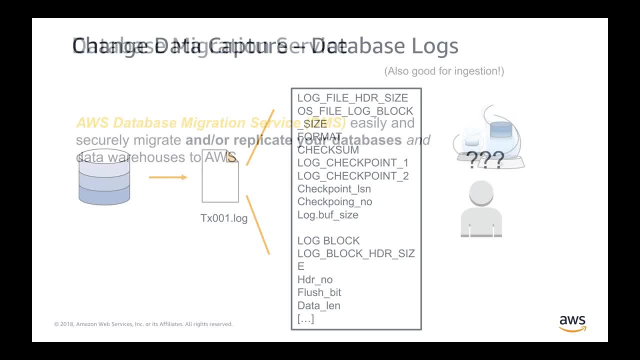 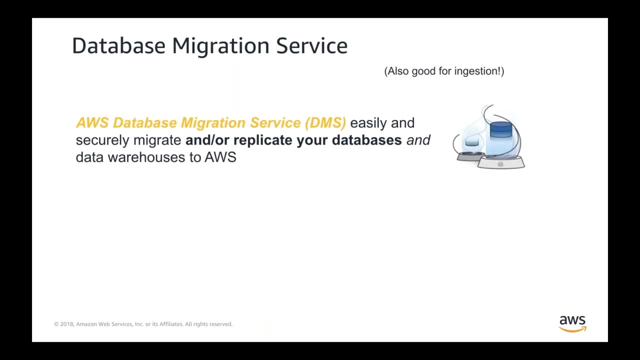 is somewhat herculean feet, prone to error and a major source of data inconsistencies in downstream systems due to bugs that are difficult to diagnose. introducing aws database migration service, which easily and securely migrates and or replicates your databases and data warehouses to aws dms can read your transaction logs- vendor specific transaction logs and replicate those changes into. 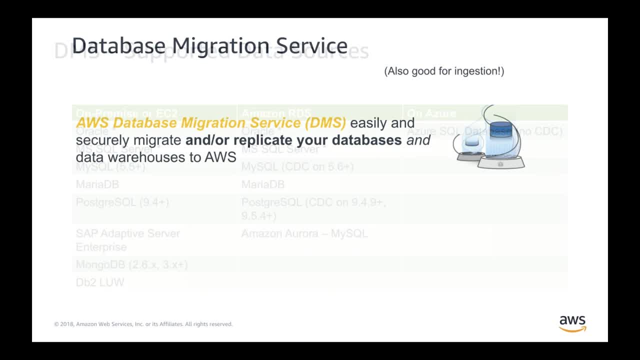 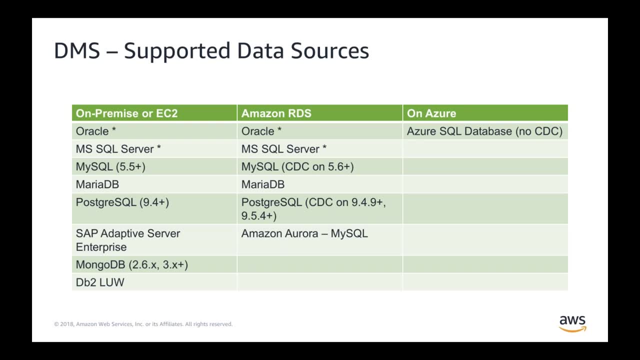 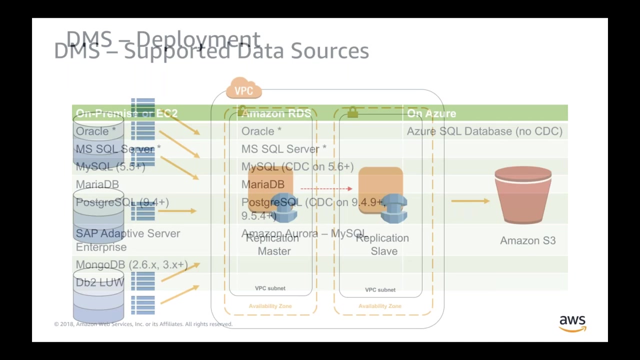 amazon s3 dms supports these databases. on on-premise it supports oracle, ms sql server, mysql, maria db or postgres. on rds it supports all the favors, including amazon, aurora, mysql and on azure it supports the azure sql server as well database. it doesn't support cdc on the sql database. cdc is the change data capture system by leading the 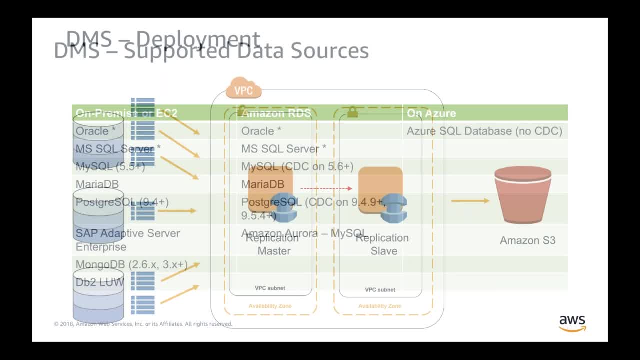 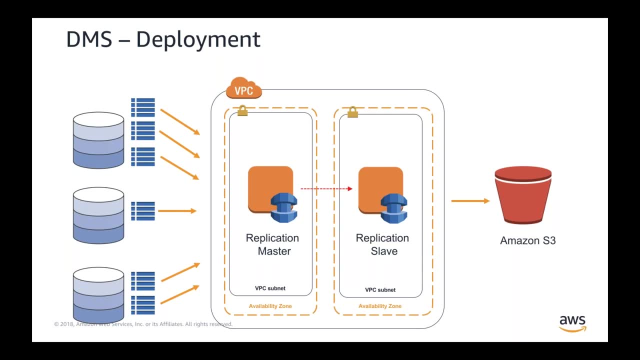 transaction logs and processing it when you deploy dms. you can deploy dms in a multi-az environment which has application master and a replication slave. this ensures that your replication is constant and is is not affected due to an availability zone not being available or underlying hardware issues. your database. 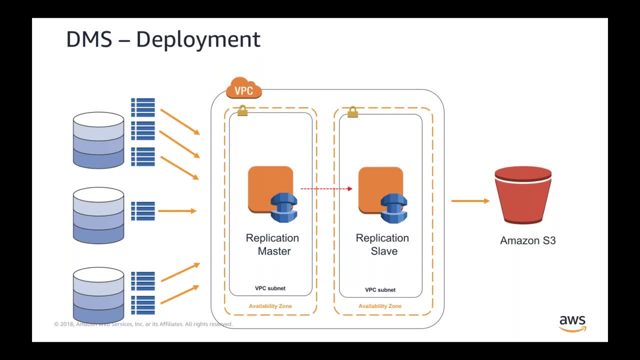 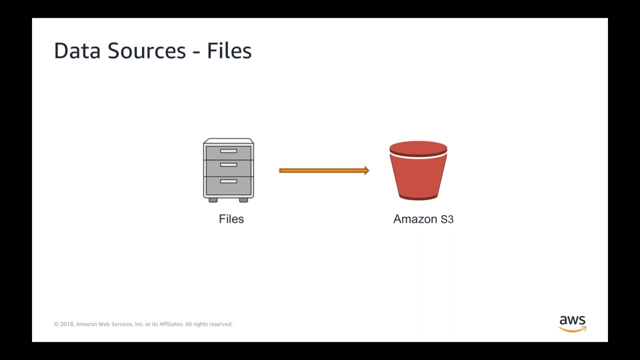 collection logs are read by the replication master and they are processed and delivered to amazon s3. amazon s3 is your data lake, where your data is stored. next let us look at files. to get files into aws, first you need to decide whether you're going to transfer them over a network or offline. this really depends on the overall size of the 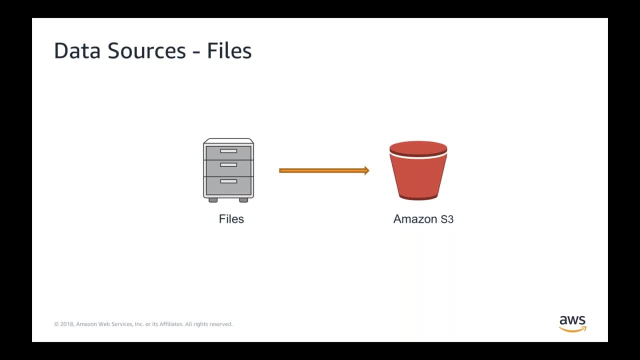 files being transferred, the window of time you have to transfer them- you need to continuously transfer new files and changes- and how much you want to spend For smaller total volumes of data. you can transfer these files over the internet. If you want some extra security, you can use a VPN To get the best line speed and isolation. 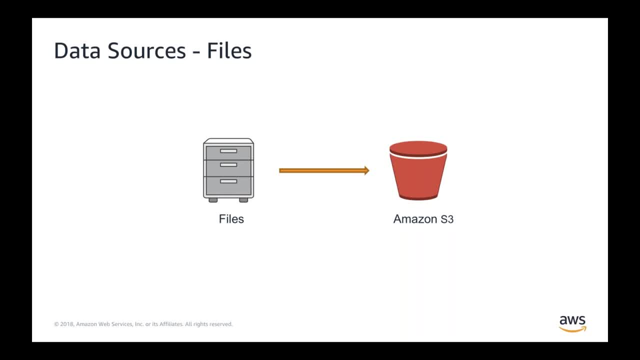 you can opt to fire up a direct connect circuit. Another option to get faster speeds is to send your files through one of the AWS edge locations, getting you onto AWS network faster and reducing the total number of hops Once your connection is set up. there is a number. 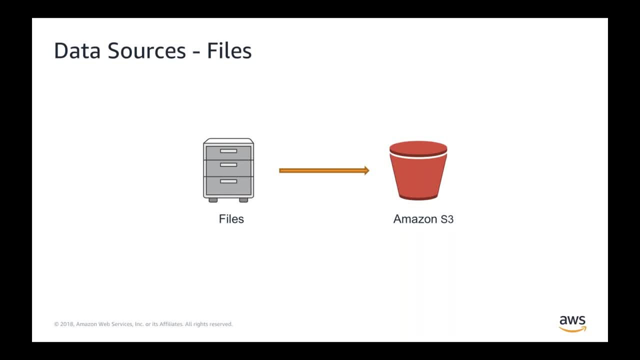 of tools and services out there that can help with transferring your files. We provide file gateway as one option. If you have too much data and not enough time, you could elect to physically ship your data to AWS via one of our snowmobile or snow star options that. 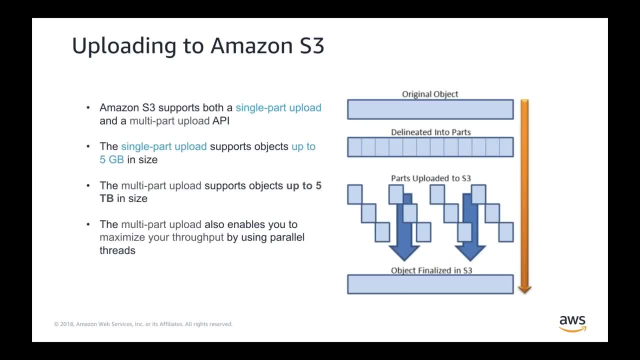 we have Uploading your data to Amazon S3. As I mentioned can be done via a direct connection to S3 and using the S3 APIs to do multi-part uploads of files beyond 5GB in size. You can. S3 supports up to five terabyte. 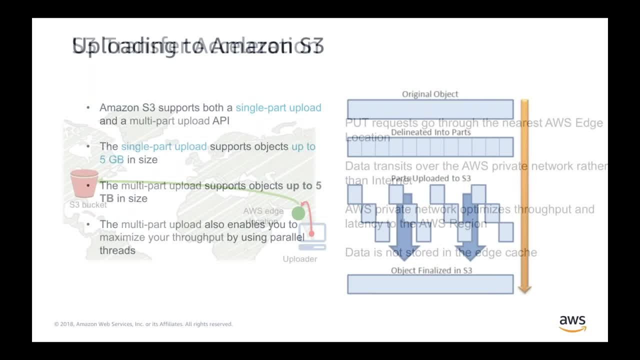 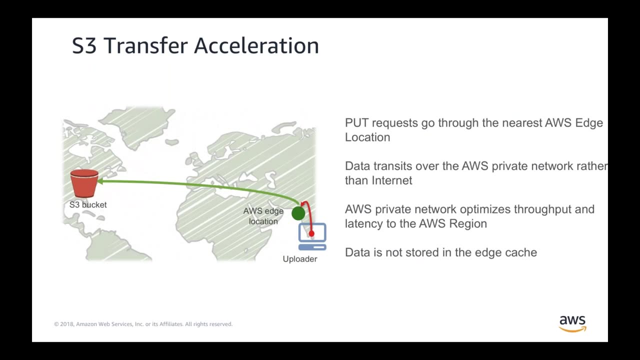 in size for a single object. The multi-part upload also enables you to maximize your throughput by using parallel threads. You can also use S3 transfer acceleration to put requests to go through the nearest AWS edge location. Data transits over the AWS private network rather than the internet. AWS private network optimizes throughput and 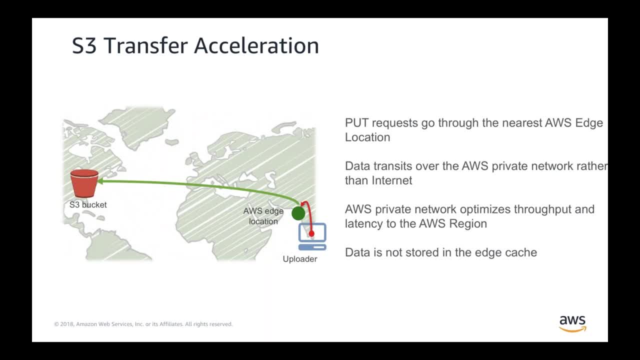 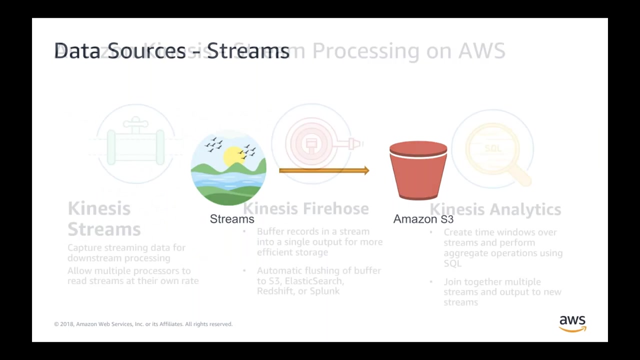 latency to the AWS region. Data is not stored on the edge caches. The edge caches are used only as a transit point to send your data onwards to S3 at the lowest latency and hops possible. Streams- Streams are becoming very critical these days. Your streams originate from clickstream. 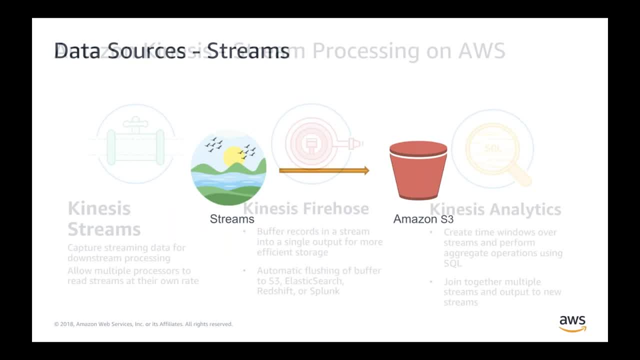 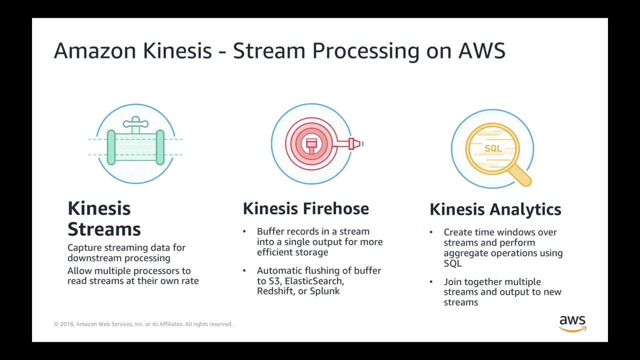 data can originate from IoT data, as discussed earlier. So what services that AWS provide for stream processing and stream delivery? Kinesis Stream is the stream processing service on AWS. It has three distinct services: Kinesis Data Streams, which capture streaming data for downstream processing. 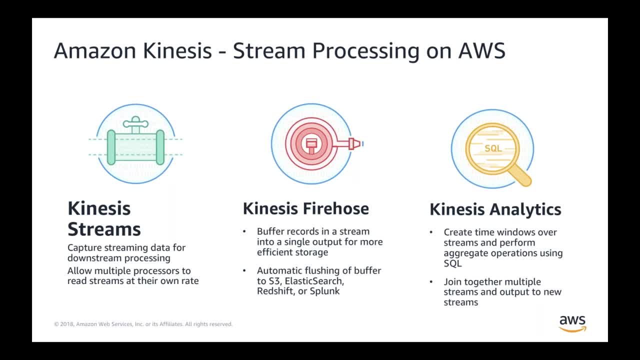 Kinesis Data Firehose for buffering records in a stream and delivering it into S3. Elastic Search, Redshift or Splunk. Kinesis Analytics is used for doing analytics on the streaming data. You may want to perform aggregate operations using SQL. You can join multiple streams and 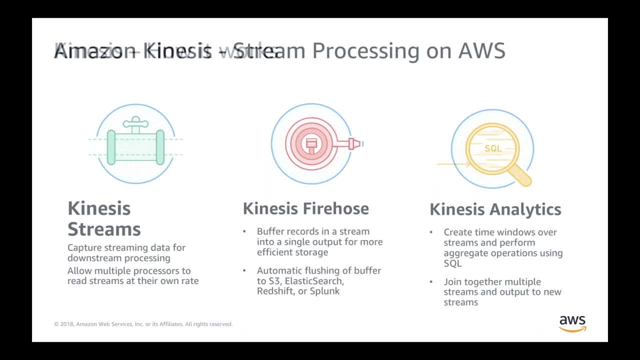 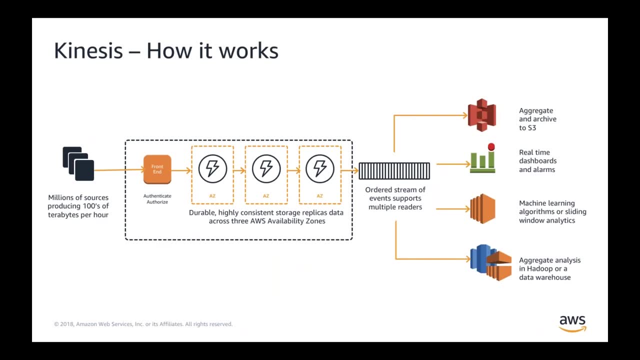 output to a new stream as well. So let us see how Kinesis works today. Millions of sources producing hundreds of terabytes of sql data. We find that it does not have 네 So Freelance, 메 소 slash- Hey, I mean Agile. you can find and pull out a lot of other objects, such as 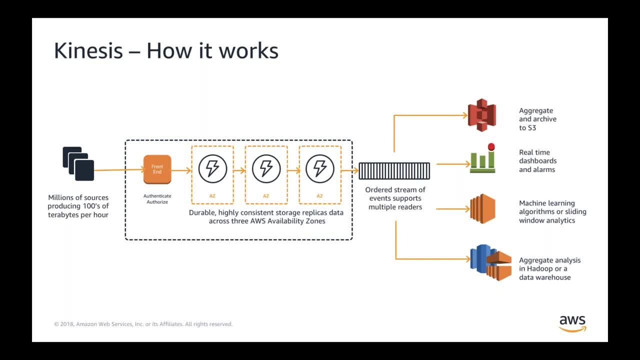 Harry Potter After hasn't been labelled. Definitely one of theniej Sérieuse. It takes a while, But there are plans for this. We hope you're王 read from that bookmark as well. You can aggregate an archive to S3.. You can create real-time. 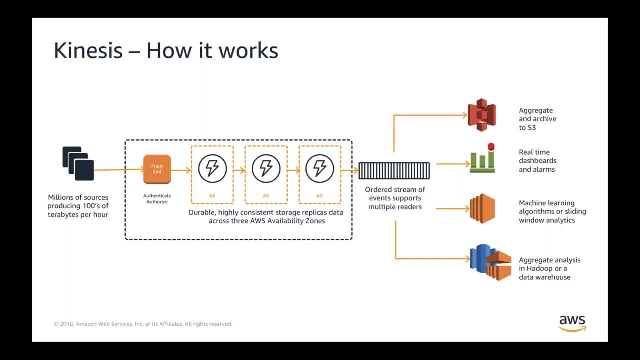 dashboards and alarms. You can also do machine learning algorithms or sliding window analytics using Kinesis Analytics or aggregate analytics in Hadoop or a data warehouse. You can do something like Spark streaming on data coming in from Kinesis Streams. The third source is logs. 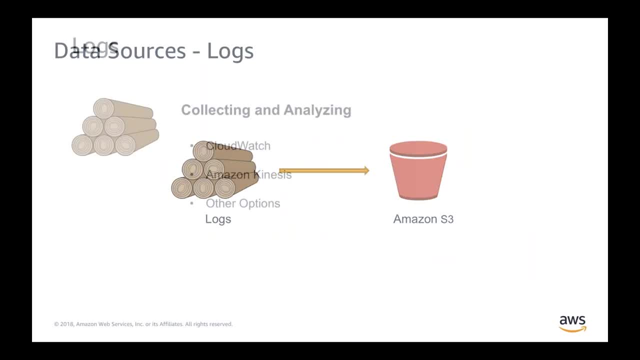 Logs are generated everywhere in your data center on your EC2 instances. today, How do I take these logs into Amazon S3, which is going to be my centralized space for doing analytics? You can collect and analyze logs using CloudWatch. You can use Amazon Kinesis or other options like. 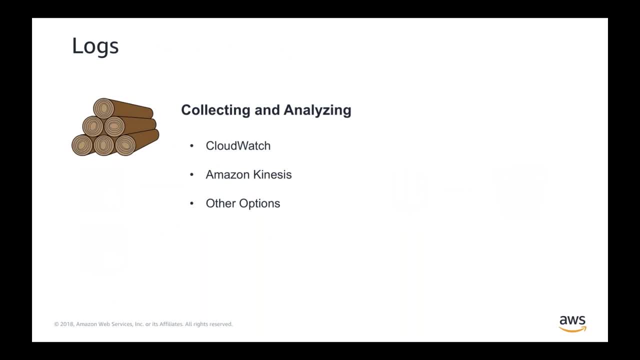 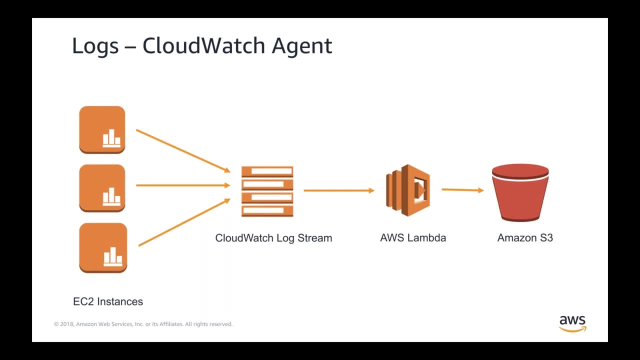 Fluentd, which can allow you to aggregate data and stream it onto S3.. The CloudWatch logs basically take data from ec2 instances by running easy agents on these ec2 instances to get the data into a cloud watch log stream. you can use lambda to 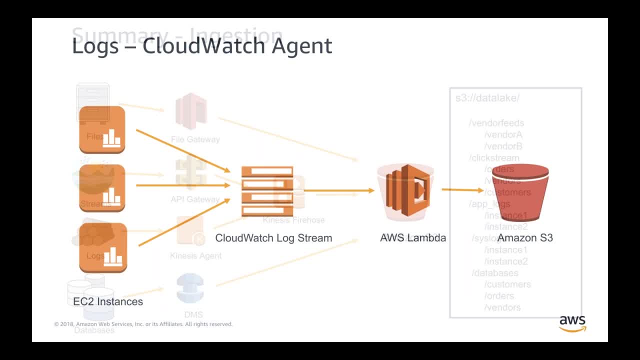 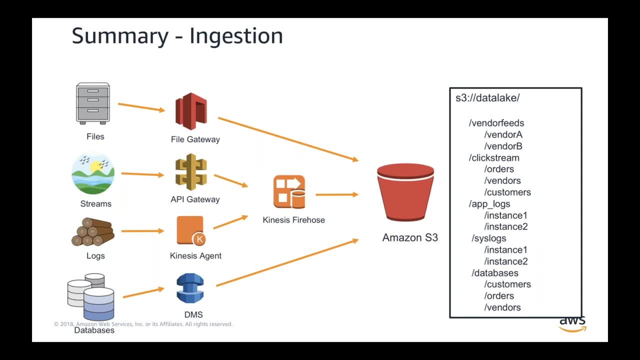 process the data and store it on an s3 bucket. in summary, your ingestion mechanisms on to the data lake looks like this: your files coming through a file gateway into Amazon s3. you have streams using API gateway to kinesis firehose. logs using kinesis agents into kinesis firehose, which ends up into the. 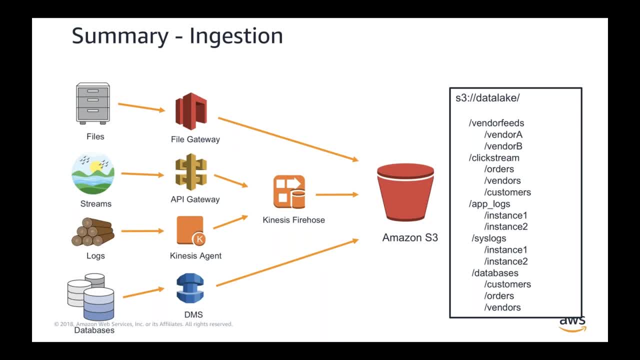 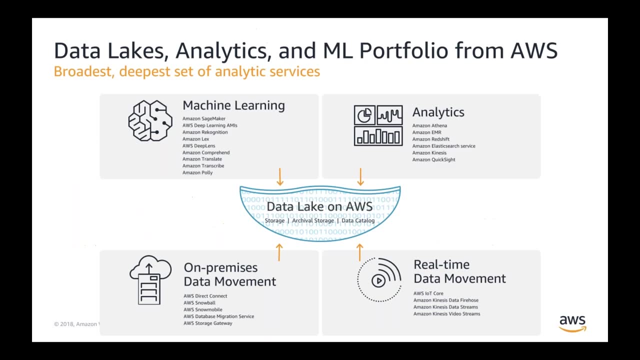 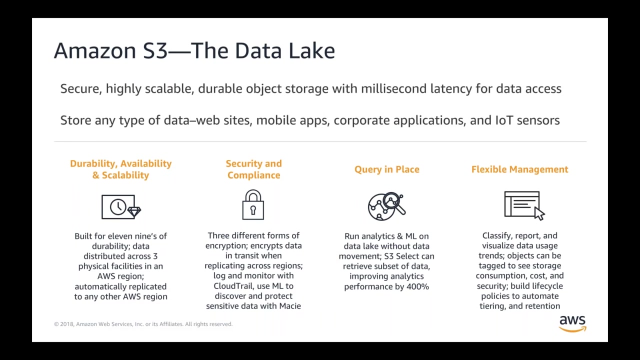 s3 data lake. you have DMS, which takes transaction logs from databases, processes them and puts them in the Amazon s3 bucket as well. this is the process of hydrating your data lake. so what is the data lake on AWS? Amazon s3 is the data lake. it is secure. 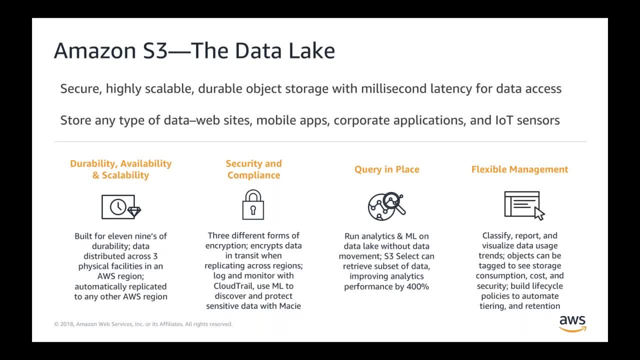 highly available durable object store with millisecond latency for data access. it has unmatched durability and availability and scalability. Amazon s3 runs on the world's largest global cloud infrastructure and is designed from the ground up to deliver 11 nines of durability data and Amazon s3 standard, s3 standard IA and Amazon glacier storage classes. 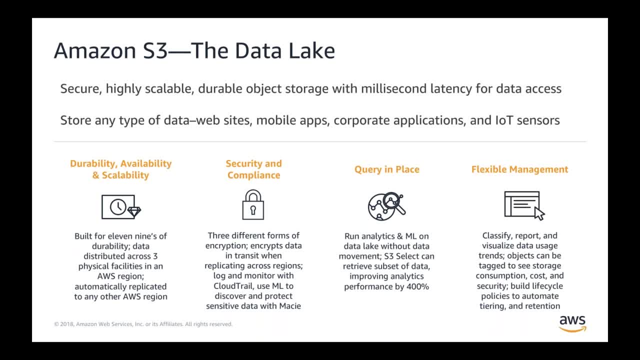 is automatically distributed across a minimum of three physical availability zones that are typically miles apart within an AWS region. the Amazon s3 one zone IA storage class stores data in a single AZ and is ideal for customers who want to lower cost options for infrequently access data and do not 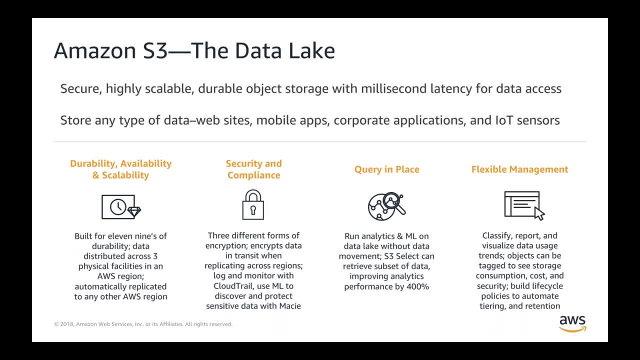 require the availability and resilience of s3 standard storage. Amazon s3 can also automatically replicate data to any other AWS region. it has the most comprehensive security and compliance capabilities. s3 supports three different forms of encryption. s3 offers sophisticated integration with AWS cloud trial to log, monitor and retain storage API call. 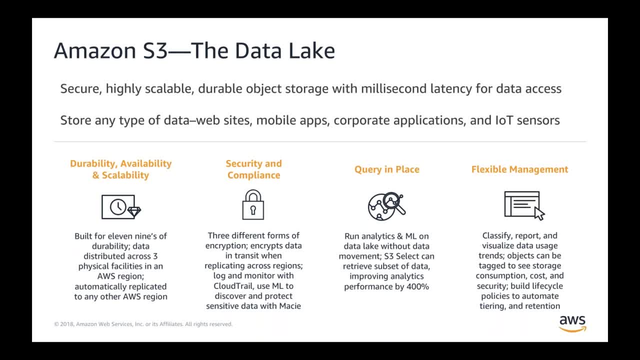 activities for auditing. Amazon s3 is the only cloud storage platform with Amazon Macy which uses machine learning to automatically discover, classify and protect sensitive data in AWS. s3 supports security standards and compliance certifications, including PCI, DSS, HIPAA, high-tech FedRAMP, EU data production directive and FISMA, which can 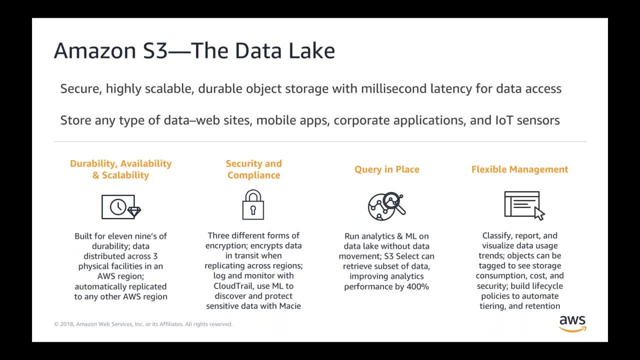 help customers satisfy compliance requirements for virtually every regulatory agency around the globe. Amazon s3 also allows you to run sophisticated big data analytics on your data without moving the data into a separate analytic system. Amazon Athena, which we will talk about in a few slides, gives anyone who knows sequel on-demand query access to vast amounts of. 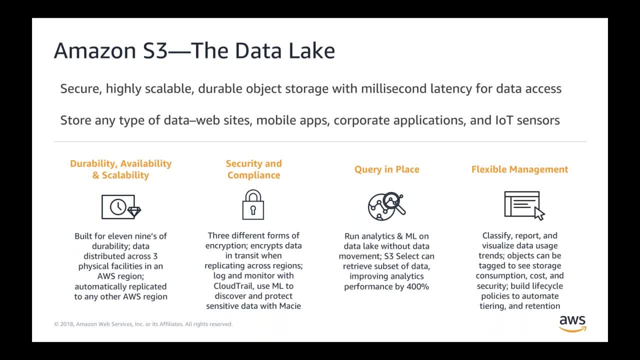 unstructured data. Amazon redshift spectrum lets you run queries spanning both your data warehouse and industry, and only AWS offers Amazon s3. select a way to retrieve only the subset of data you need from an s3 object, which can improve the performance of most applications that frequently access data. 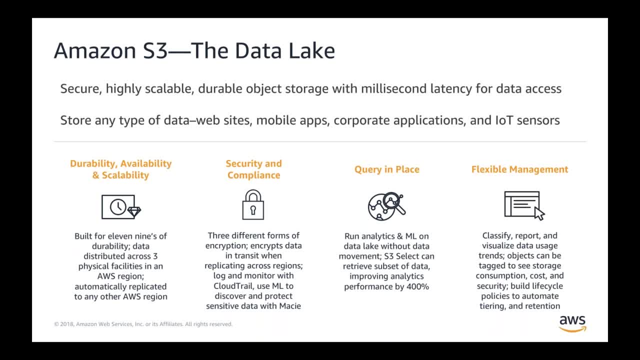 from s3 by up to four hundred percent. Amazon s3 offers the most flexible set of storage management or administration capabilities. storage administrators can classify, report and visualize data usage trends to reduce costs and improve service levels. objects can be tagged with unique, customizable metadata so customers can see and control storage. 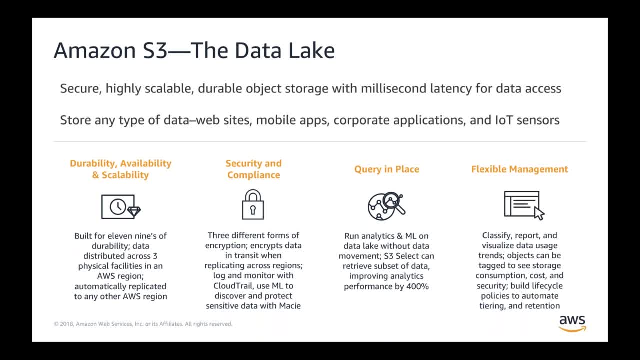 consumption, cost and security separately for each workload. the s3 inventory feature delivers scheduled reports about objects and their metadata for maintenance, compliance or analytics operations. s3 can also analyze object access patterns to build lifecycle policies that automate tearing, deletion and retention. since Amazon s3 works with 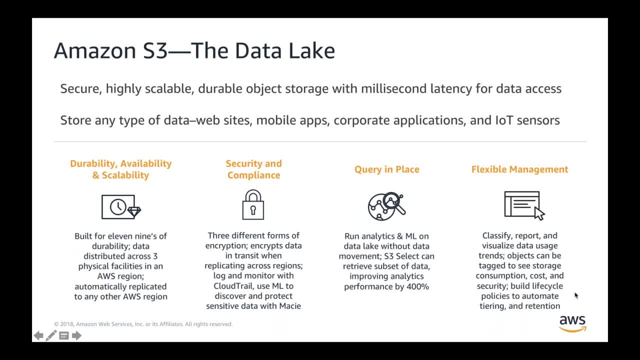 AWS lambda, customers can log activities, define alerts and invoke workflows, all without managing any additional infrastructure. data can be stored in the s3 data тай游户中的文件中的数据中的材料和单vio数据组成效 Lake, and can be backed up into Glacier and used for archive purposes. It is secure, durable and 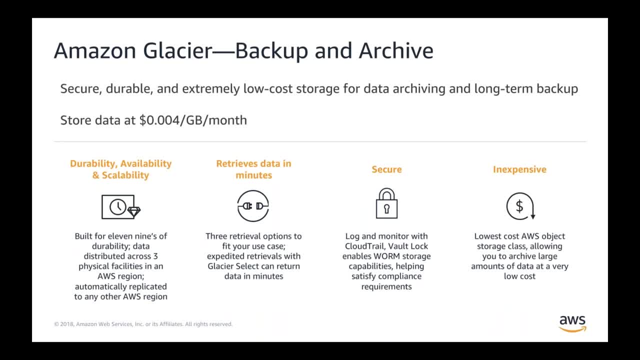 extremely low-cost storage for data archiving and long-term backup. Retrievals are as quick as one to five minutes, Unmatched durability and scalability built on the same principles of Amazon S3, and it gives you the most comprehensive security and compliance capabilities as well. 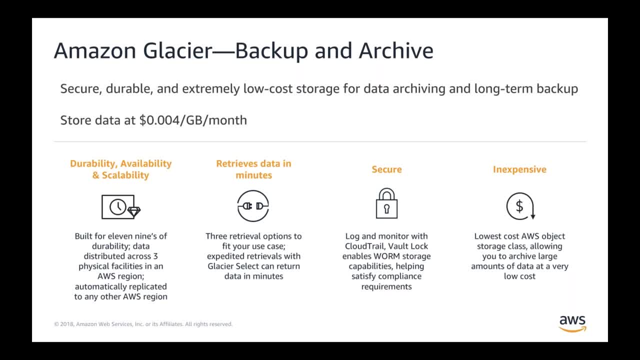 On top of all this, it is a low-cost service. It's designed to be a lower cost for you to store your archive data in Amazon Glacier, and you can use Amazon Glacier to pay only for what you need, with no minimum commitments or upfront fees. Storage is not enough. Data needs to be discoverable. 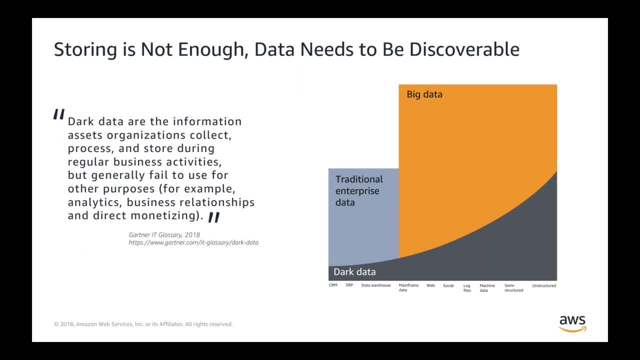 Gartner defines dark data as the information assets that organizations collect, process and store during regular business activity, but generally fail to use other purposes, like in analytics, business relationship and direct monetization. Storing and securing this data typically incur more expense than they do value. We are seeing as more organizations collect large 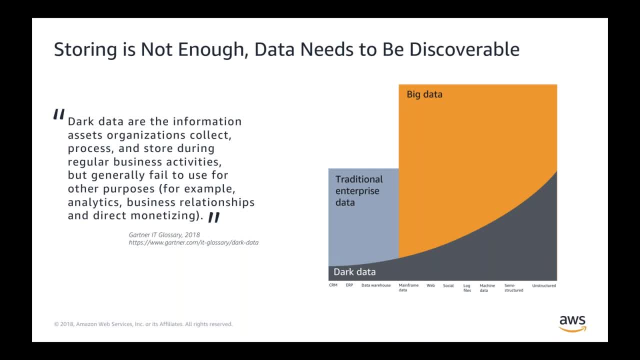 amounts of data as characteristics in a big data and data-like workloads, and we see this as a major challenge for the organization. The dark data grows with the amount of data stored. This is a challenge if the data stored is not easily discoverable to the end users. Users need to be aware of what data is there. 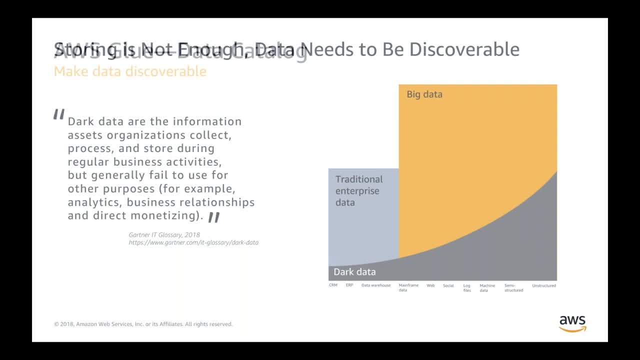 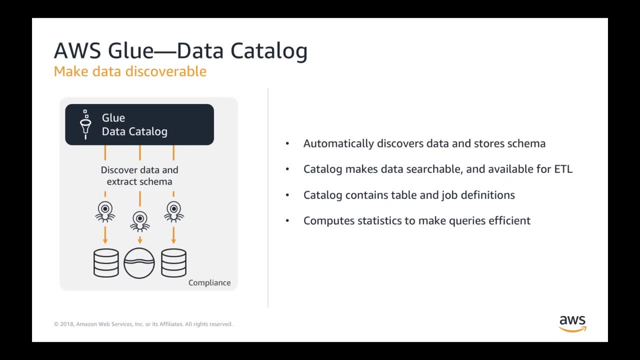 so that they can do analytics on that data. AWS Glue, apart from being an ETL service, is also a data catalog. It makes data discoverable. It thus minimizes dark data in your organization. The AWS Glue data catalog is your persistent. 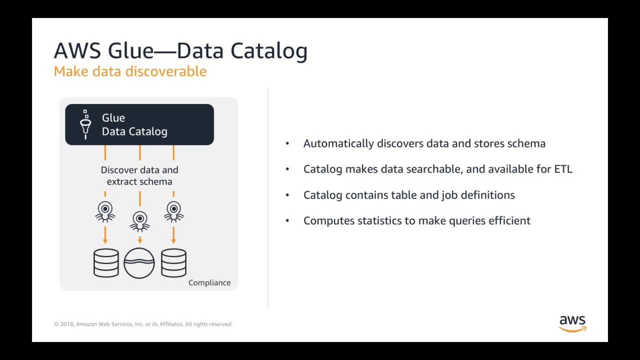 metadata store for all your data assets, regardless of where they are located. The data catalog contains table definitions, job definitions and other control information to help you manage your AWS Glue environment. AWS Glue crawlers connect to your source or target. data store progresses through a prioritized list of classifiers to determine the schema. 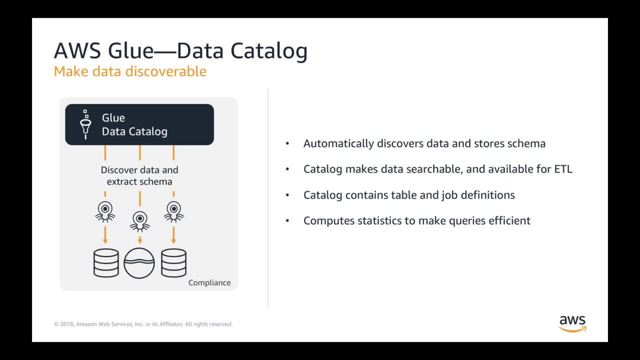 for your data and to manage your data collection. You can access any data in your organization's and then creates metadata in your AWS Glue data catalog. This metadata is stored in tables in your data catalog and used in authoring process of your ETL jobs. 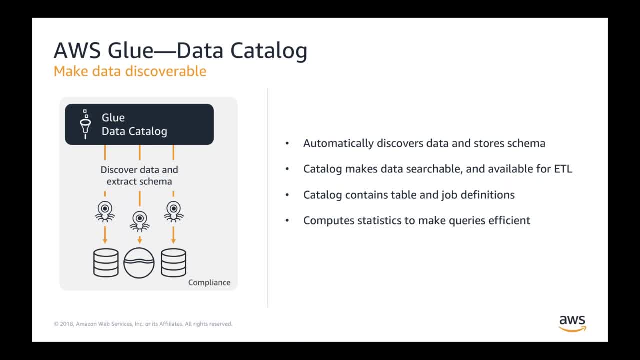 You can run crawlers on a schedule on demand or trigger them based on an event to ensure that your metadata is up to date. It automatically computes statistics and registers partitions to make queries against your data efficient and cost effective. It also maintains a comprehensive schema. version S3. 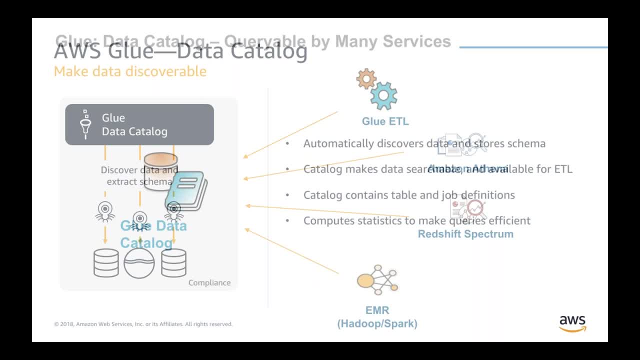 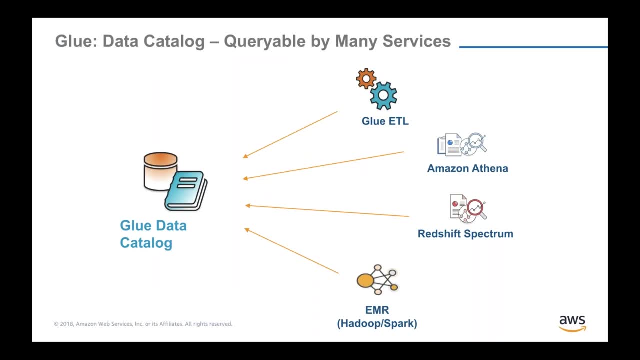 so you can understand how your data has changed over time. The Glue data catalog can be shared by many services. We spoke about Glue ETL that can use the Glue data catalog to run your transformations. Amazon Athena can use the Glue data catalog. 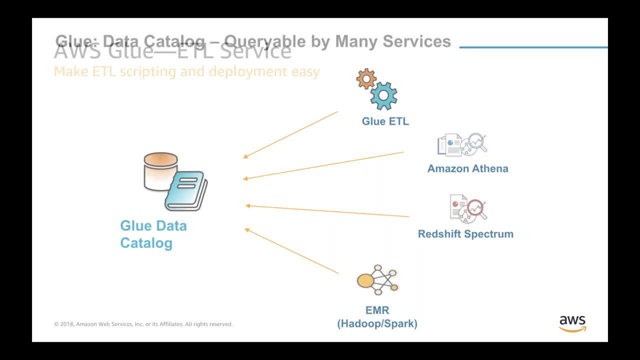 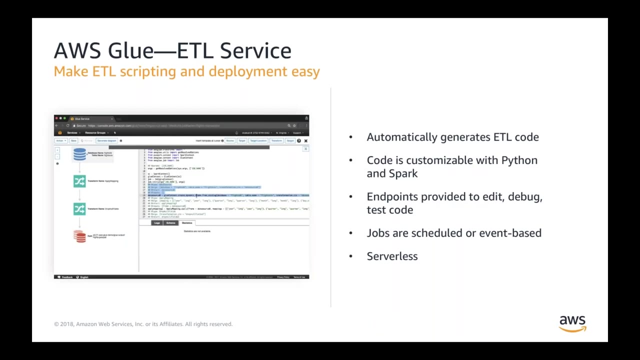 for querying the S3 buckets. Redshift Spectrum can use the Glue data catalog and earmarked. You can also use the Glue data catalog as a high metadata store. Glue also runs an ETL service which makes it easy for you to do scripting and deployments. 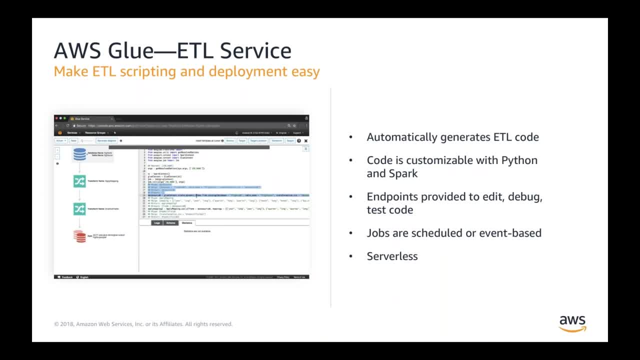 It automatically generates ETL code to extract, transform and load your data. Simply pointing your Glue scripts to a data source and target Glue creates ETL scripts to transform, flatten and export. It also generates ETL code to generate and enrich your data. 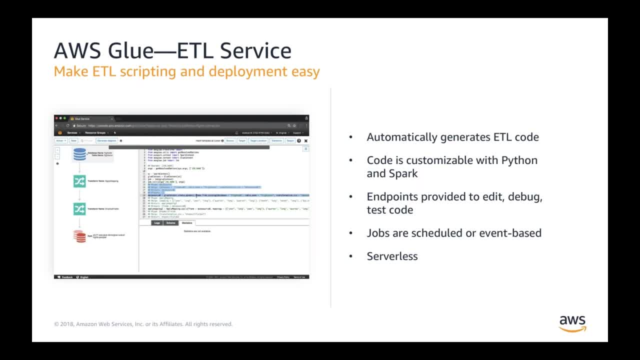 The code is generated in Python and written for the Apache Spark 2.1 environment. This also lets you edit the code. Glue provides development endpoints for you to edit, debug and test code it generates for you. You can use your favorite IDE or notebook. 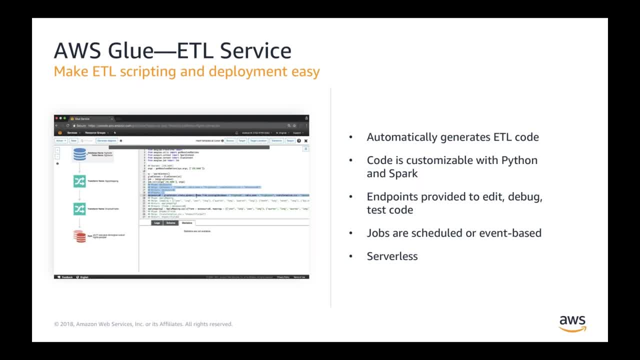 You can write custom readers, writers or transformations and then import them into your ETL job as custom libraries. Finally, when your code is complete, you can schedule recurring ETL jobs and then import them into your ETL job as custom libraries. 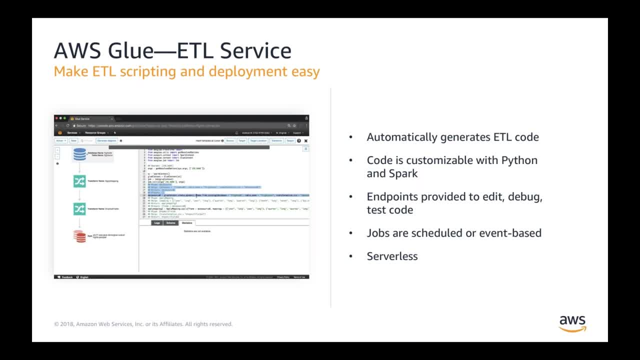 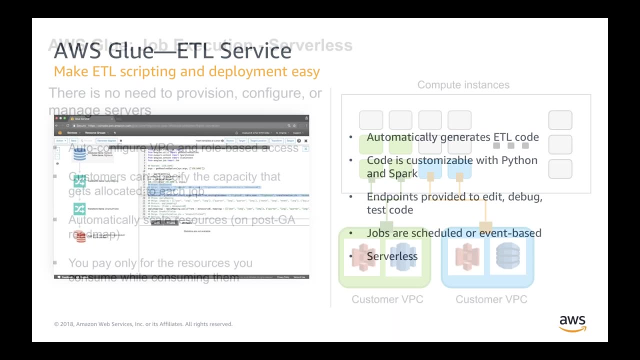 Finally, when your code is complete, you can schedule recurring ETL jobs chain, multiple jobs together or invoke jobs on demand from other services like AWS Lambda, AWS Glue. Lambda and AWS Glue manages the dependencies between your jobs. automatically scales underlying resources. 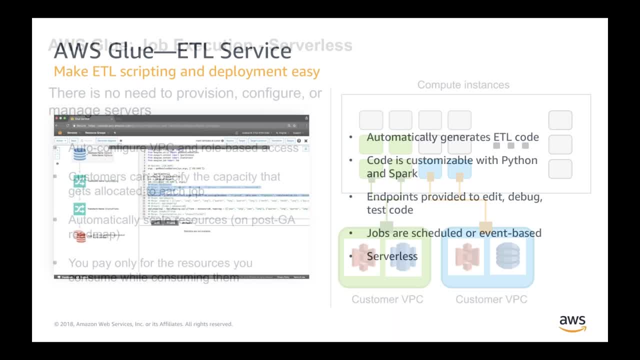 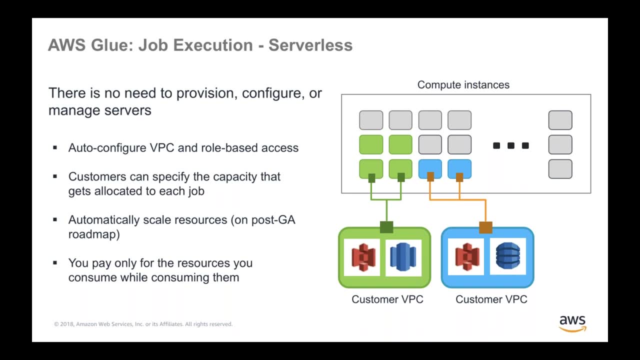 and retries jobs if they fail. The AWS Glue job execution is serverless. There is no need for you to provision, configure or manage servers. It auto-configures VPC and role-based access. Customers need to be able to use it. 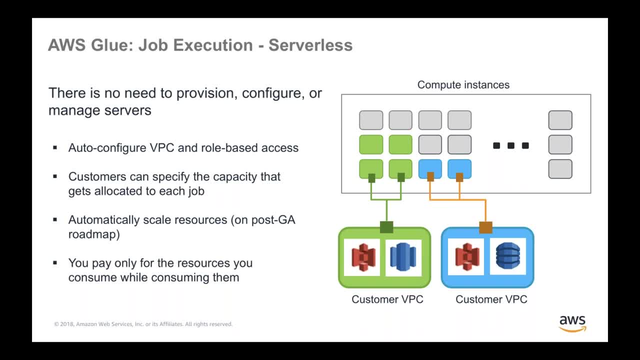 Customers can specify the capacity that gets allocated to each job. We also have it on the roadmap to provide you the ability to scale your resources based on the time that you want your bad jobs to run. You only pay for resources you consume while consuming them. 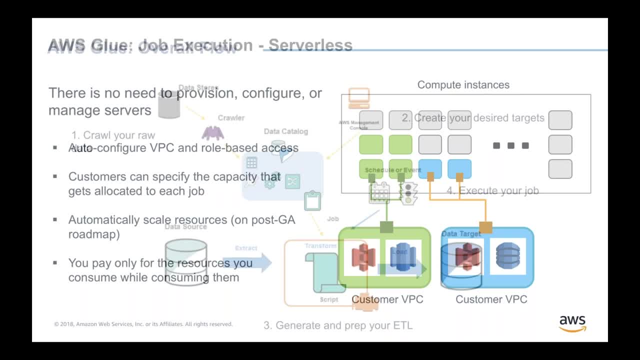 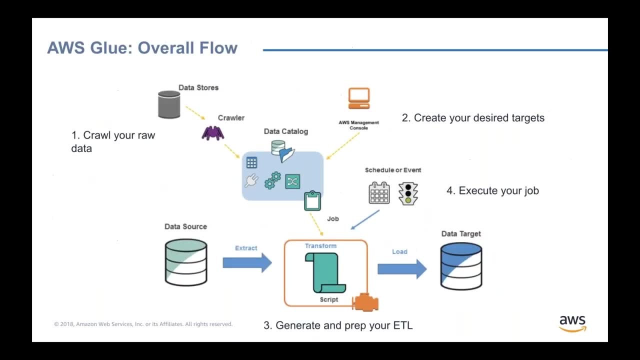 It does not intermingle data within customers or within jobs. They all run in isolation on warm pool clusters that we have defined. So the overall flow for Glue is: first: crawl your raw data, create your data catalog. Once you have created your data catalog, 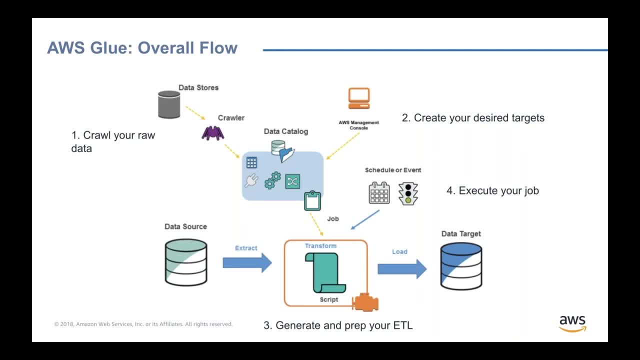 you go ahead and create your desired targets, the load part of your ETL pipeline, And then you would generate and prep your ETL jobs. You may use Glue provided methodologies to generate code, or you may want to write your own code and then deploy the code on the Glue platform. 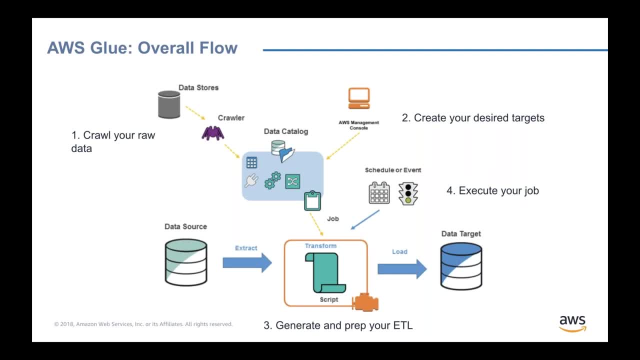 Once it has been deployed, you schedule your jobs based on event times or based on events that are happening in your system. So the jobs extract the data from the data stores from where we have crawled them, transforms them and loads them into the data target. 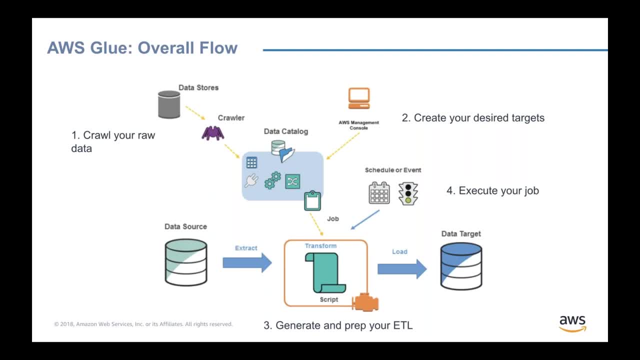 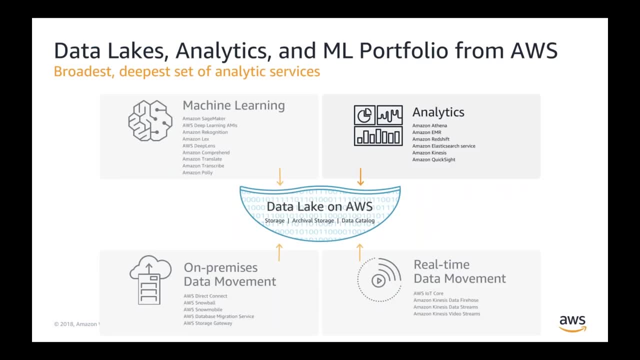 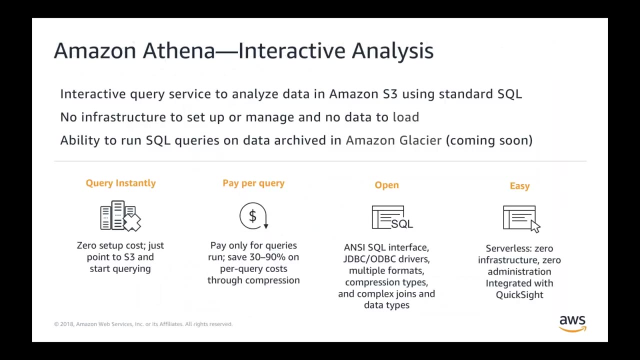 Glue is a fully managed environment for your ETL and to run your ETL at scale. Next, let us look at what analytics that AWS provides on the data lake for you. Amazon Athena is an interactive analysis service that makes it easy to analyze. 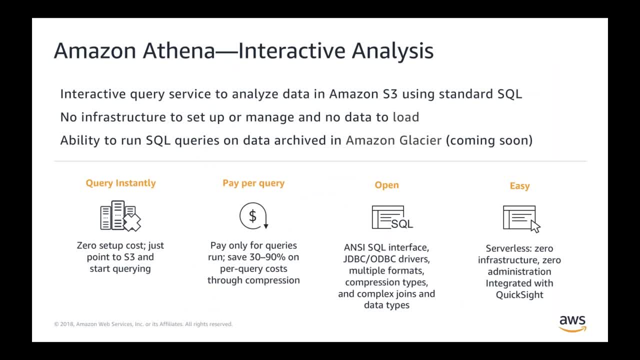 data in Amazon S3 using standard SQL. Athena is serverless, so there is no infrastructure to manage and you pay for only the queries that you run. Athena is easy to use: You just have to simply point Athena to your S3 buckets. 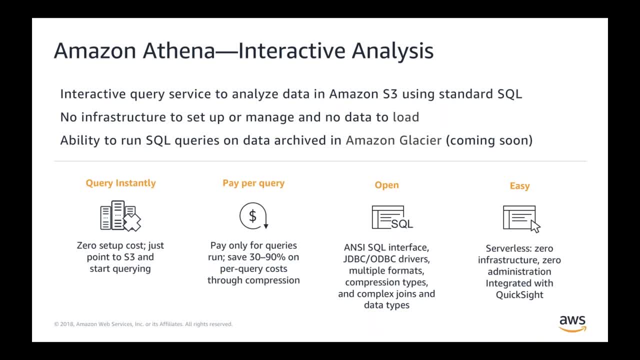 define the schema and start querying using standard SQL. Most results are derived within seconds With Athena. there is no need for complex ETL jobs to prepare your data for analysis. This makes it easy for anyone who knows SQL to start looking at the data. 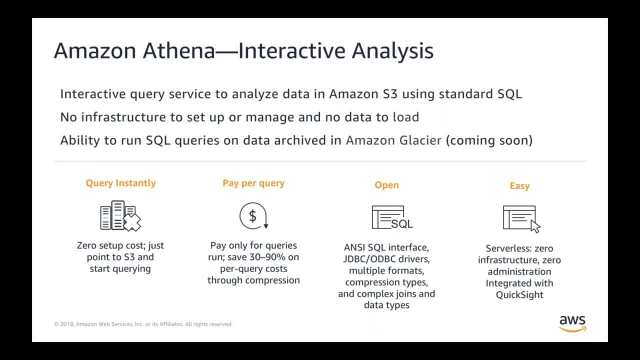 and doing analysis on the data. Athena is out-of-the-box integrated with AWS Glue data catalog, allowing you to create a unified metadata repository across various services, crawl data sources to discover schemas and populate your catalog with new and modified table and partition. 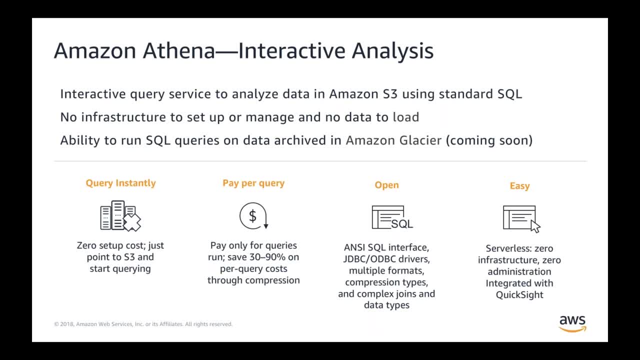 definitions and maintain schema versioning. Since there are no servers, you can quickly query your data without having to set up, manage any servers or data warehouses. Just point to your data in Amazon S3, define the schema and start querying using the built-in. 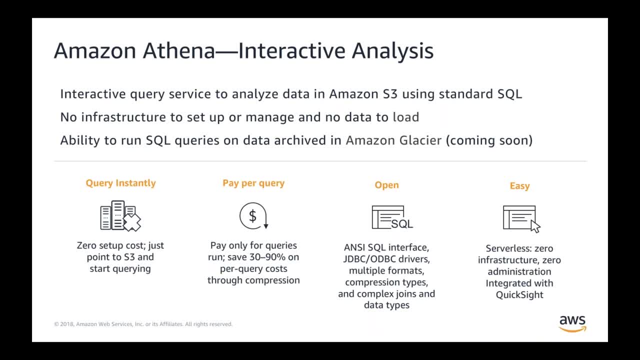 query editor Only for pay for data scanned, While Amazon Athena you pay only for the queries that you run. You are charged $5 per terabyte scanned by your queries. You can save 30-90% on your per query cost and get better performance. 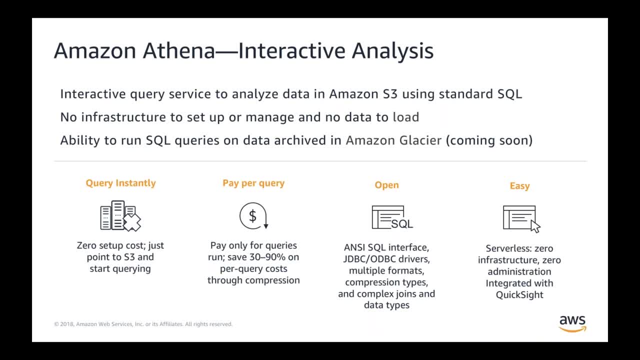 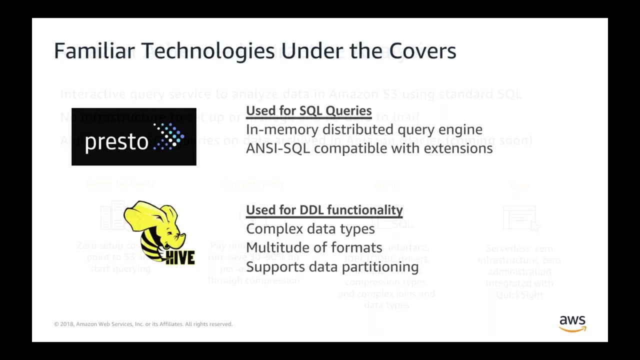 by compressing, partitioning and converting your data into a columnar format like Parquet. Athena queries data directly in Amazon S3. There are no additional storage charges beyond S3.. Amazon Athena has been built under familiar technologies. Presto is used for SQL queries. 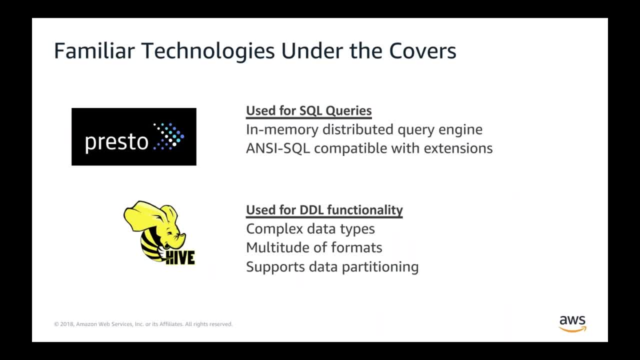 in-memory distributed query engine and C-SQL compatible with extensions. Hive metadata gives you DDL functionality, complex data types, multiple formats and also supports partitioning, As mentioned earlier. you pay per query. you pay $5 per terabyte scanned from S3.. 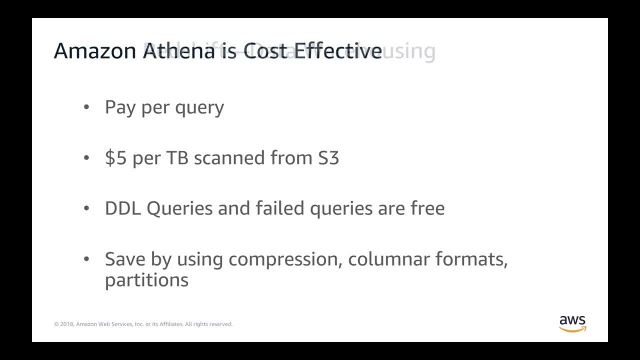 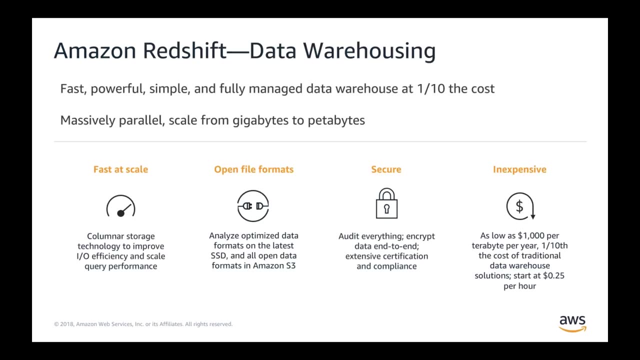 DDL queries and failed queries are not charged and you can save by compressing and using columnar formats and partitions in your data. The next service is Amazon Redshift, which is the data warehousing service. Amazon Redshift is a fast, powerful. 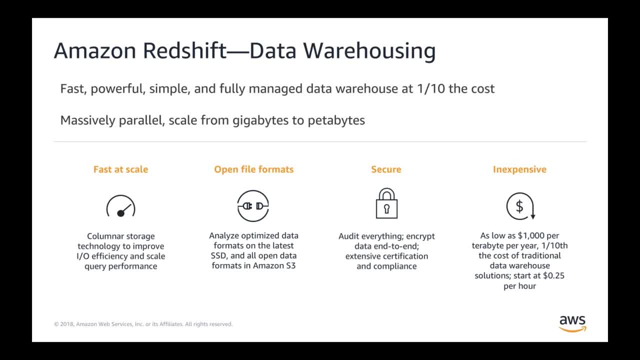 simple and fully managed data warehouse at one-tenth the cost. It is cost-effective to analyze all your data using standard SQL and use existing business intelligence tools. It allows you to run complex analytics queries against petabytes of structured data using sophisticated query optimizing. 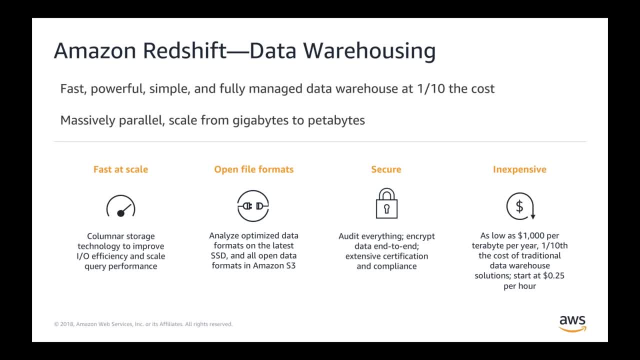 columnar storage on a high-performance local disk and massively parallel query execution. Most results come back in seconds. With Amazon Redshift you can start small for just 25 cents per hour with no commitments and scale out to petabytes of data for $1,000 per terabyte. 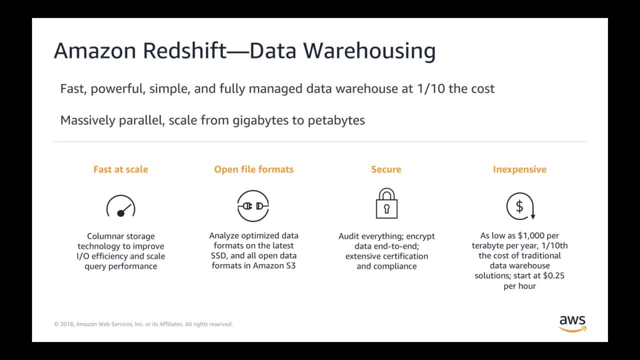 per year- less than the tenth of the cost of a traditional solution. Amazon Redshift delivers fast query performance by using columnar storage technologies to improve IO efficiencies and by parallelizing queries across multiple nodes. Data load speeds scale linearly with cluster size with integration. 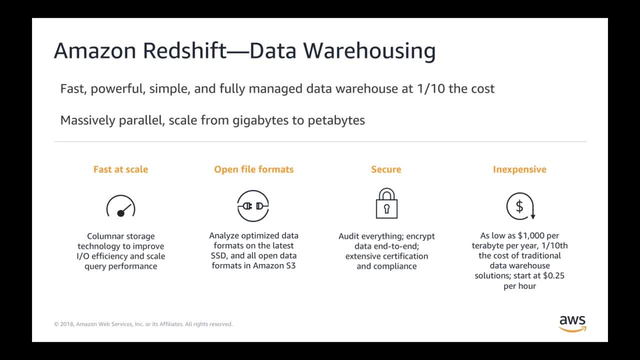 to Amazon, S3, DynamoDB, EMR, Kinesis and any SSH-enabled host. You pay only for what you use. You can have unlimited number of users doing unlimited analytics on all your data for just $1,000 per terabyte. 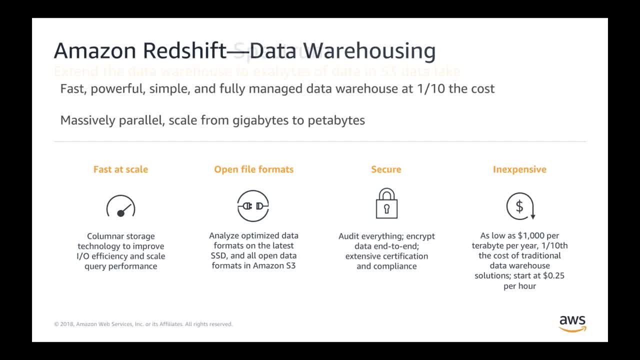 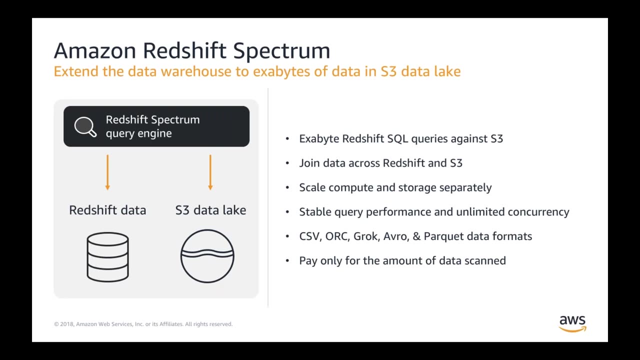 per year. Redshift Spectrum enables you to run queries against exabytes of data in Amazon S3 as easily as you run queries against petabytes of data stored on local disks on Amazon Redshift. Redshift Spectrum directly queries data in Amazon S3 using the open data formats. 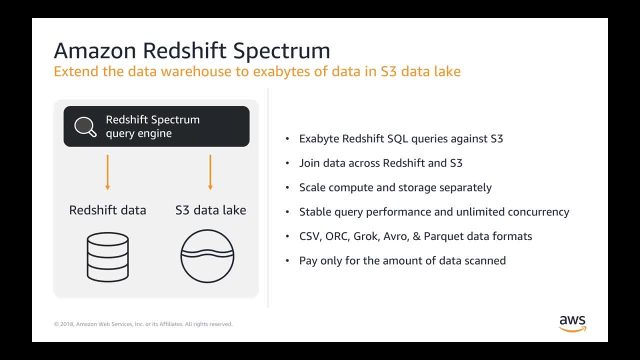 you already use, including Avro, CSV, Grok, Ork, Parquet RC files, sequence files and text files. Since Redshift and Spectrum supports the same SQL syntax, on Amazon Redshift you can run sophisticated queries using the same business. 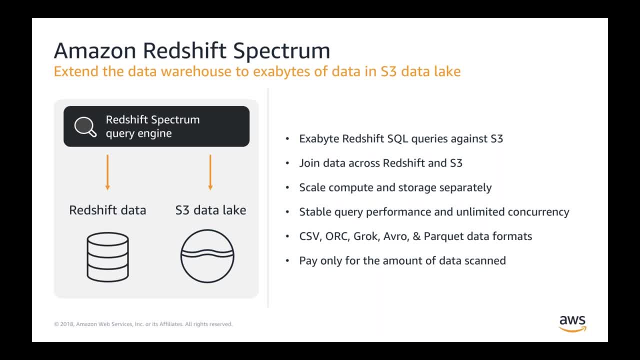 intelligence tools you use today. You can also run queries that span both the frequently accessed data stored locally in Amazon Redshift and your full data set stored in cost effectively in Amazon S3.. With Amazon Redshift Spectrum, you can start querying your data in Amazon S3. 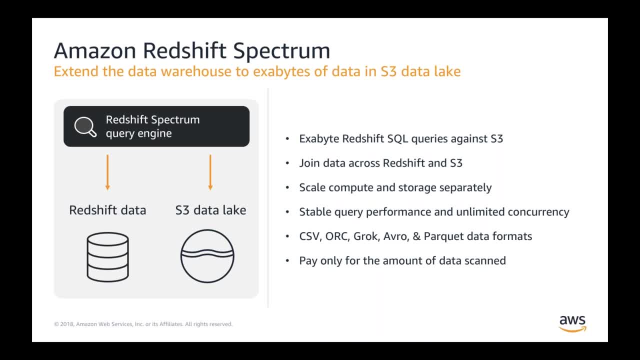 immediately, with no loading or transformation required. You just need to register your Amazon Athena, AWS Glue Data Catalog or Apache Hive Metastore. as an external schema, You can use the same SQL you use for querying Amazon Redshift tables- any BI tools that support. 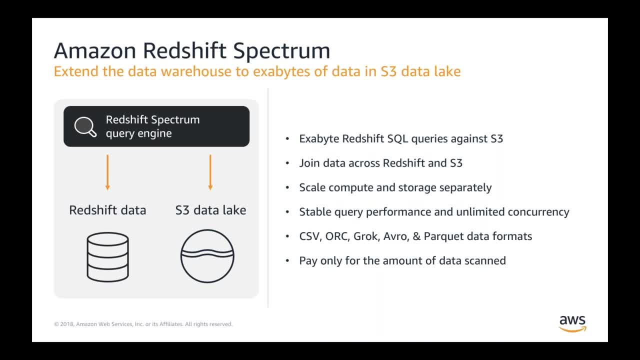 Redshift. today, Amazon Redshift delivers super fast performance. whether it is for Haddock analysis or large unstructured data sets in Amazon S3, or frequent analysis on structured data sets in Redshift tables, You can maintain hot data in your Amazon Redshift clusters to get. 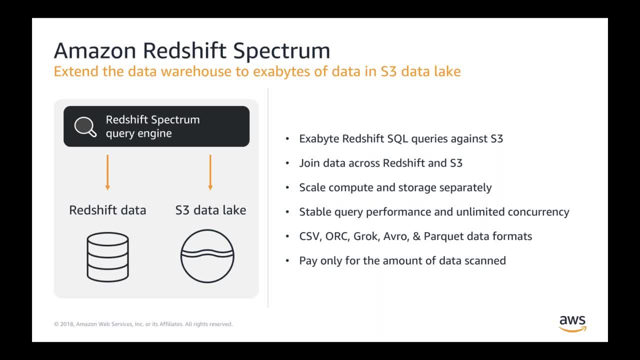 the performance of local disks and use Amazon Redshift Spectrum to extend your queries to cold data stored in Amazon S3 for unlimited scalability and low cost. The Amazon Redshift Query Optimizer will automatically determine how to minimize data scanned in Amazon S3 and the number of Redshift Spectrum. 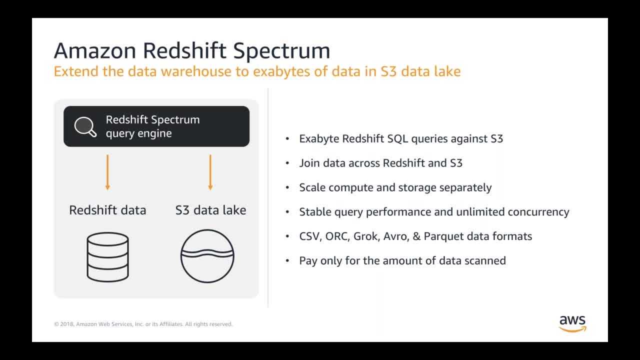 nodes to use in the query. With Amazon Redshift Spectrum, you don't have to worry about scaling your clusters. It lets you separate storage and compute, allowing you to scale each independently. You can even run multiple Amazon Redshift clusters against the same S3 data lake. 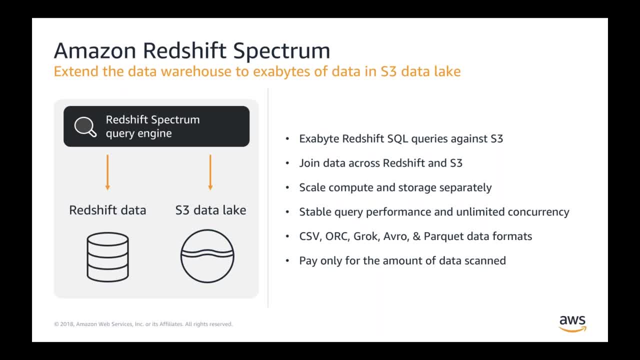 enabling limitless concurrency. Redshift Spectrum automatically scales out to thousands of instances if needed. Queries run quickly, whether processing a terabyte, petabyte or exabyte of data. As Athena, you only pay for data process. with Amazon Redshift Spectrum, You are charged $5 per terabyte. 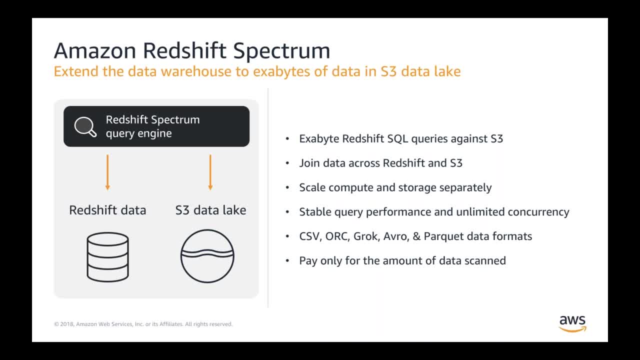 of data process to execute your query. Redshift Spectrum can query compressed data. You can save up to 30-90% on your per query cost and improve performance by compressing, partitioning and converting data to a columnar format. There are no charges for Redshift Spectrum. 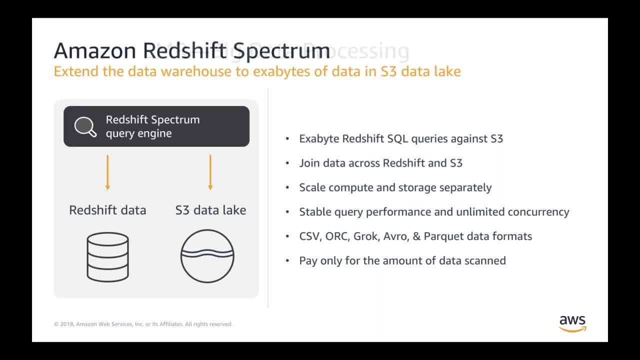 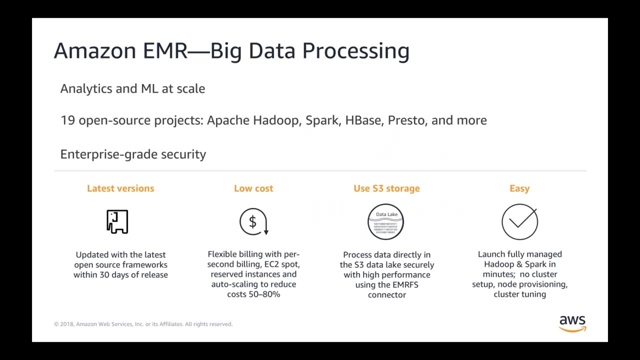 when you are not running queries. You pay standard Amazon S3 for data storage and Amazon Redshift instance rates for clusters used. Amazon EMR is for big data processing. Amazon EMR provides a managed Hadoop framework that makes it easy, fast and 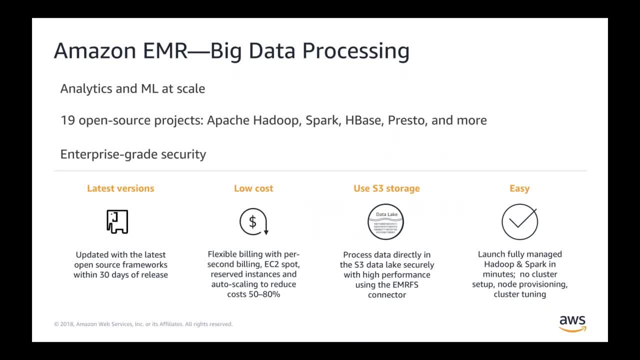 cost effective to process vast amounts of data across dynamically scalable Amazon EC2 instances. You can also run other popular distributed frameworks such as Apache, Spark, HBase, Presto and Flink in Amazon EMR and interact with data in other AWS data source, such as. 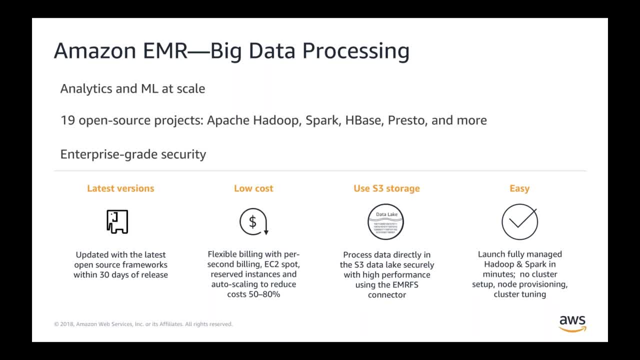 Amazon S3 and DynamoDB. Amazon EMR securely and reliably handles a broad set of big data use cases, including log analysis, web indexing, data transformations, machine learning, financial analysis, scientific simulations and bio information. We have found EMR to be one of the most. 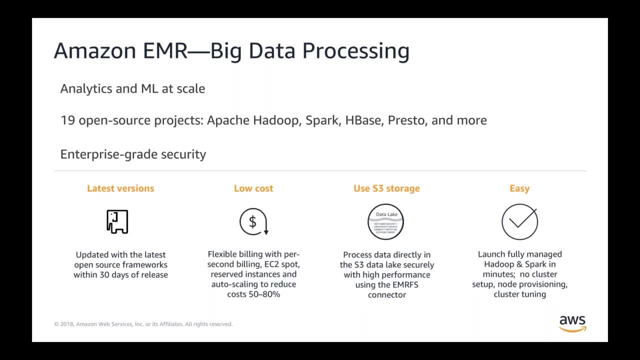 cost effective Hadoop and Spark distribution because of all the flexible ways we can bill the customer. with Persecon Billing introduced this year, We have Spark pricing that can dramatically lower your bills, or reserved instances that can lower your bill 50 to 80 percent. 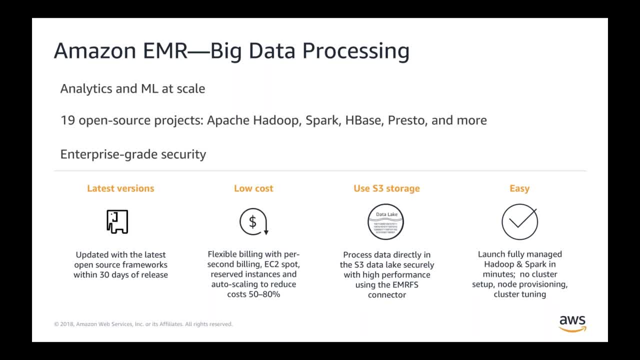 Finally, with the ability to automatically resize your clusters based on scaling rules, EMR is the most cost effective place to run Hadoop and Spark workloads. EMR clusters need not be always on clusters. They can be transient clusters with Persecon Billing, which means that. 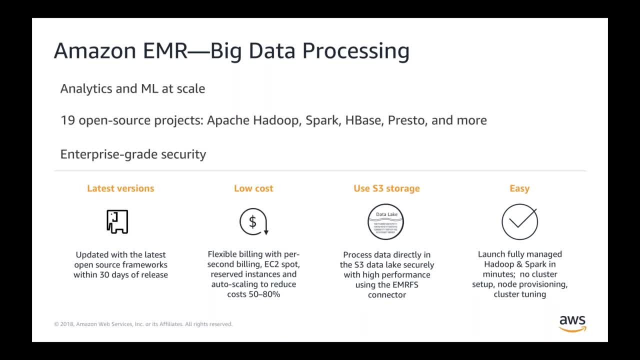 you bring up these clusters only when you want to process data and shut them down once the processing is completed. You can run multiple EMR clusters out of processing data out of the same S3 data lake, so that one can use Flink to process the data and other EMR clusters. 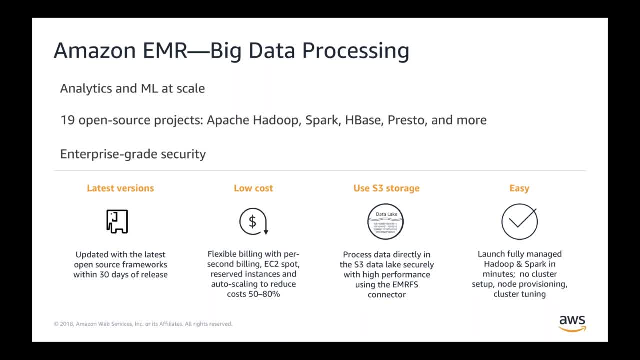 can use Spark to process the same data, So you can also launch an EMR cluster in minutes. You don't need to worry about node provisioning, cluster setup, Hadoop configuration or cluster tuning. Amazon EMR takes care of these tasks, so 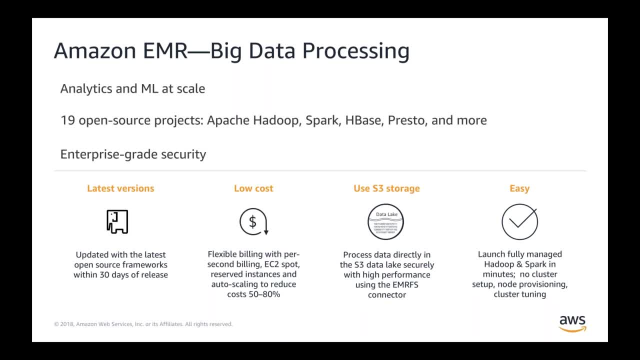 you can focus on analysis. Amazon EMR pricing is simple and predictable: You pay a per second rate for every second used. With a one minute minimum charge, you can launch a 10 node Hadoop cluster for as little as 15 cents per hour. 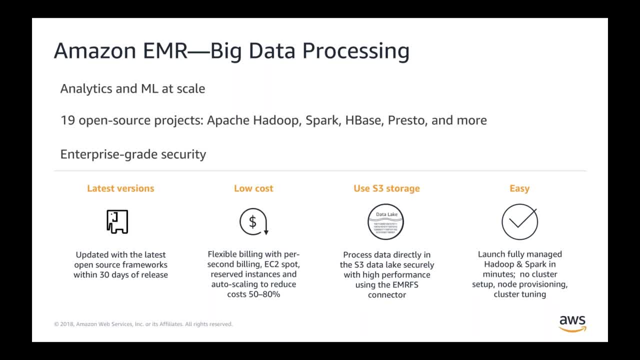 because Amazon EMR has native support for Amazon EC2 spot and reserved instances. You can also save 50 to 80 percent on the cost of the underlying instances. With Amazon EMR you can provision one hundred or thousands of compute instances to process data at any scale. 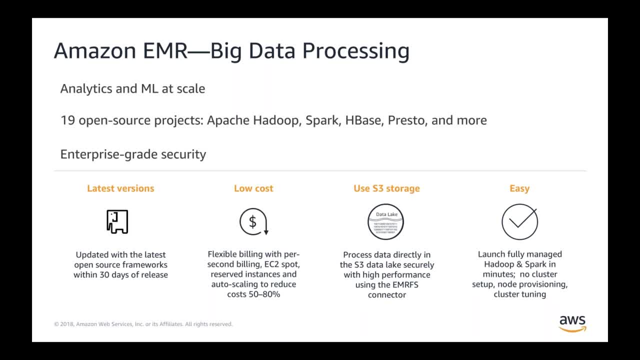 You can easily increase or decrease the number of instances, manually or with auto scaling, and you only pay for what you use. You can spend less time tuning and monitoring your cluster. Amazon EMR has tuned Hadoop for the cloud. It also monitors your cluster, retrying failed tasks and 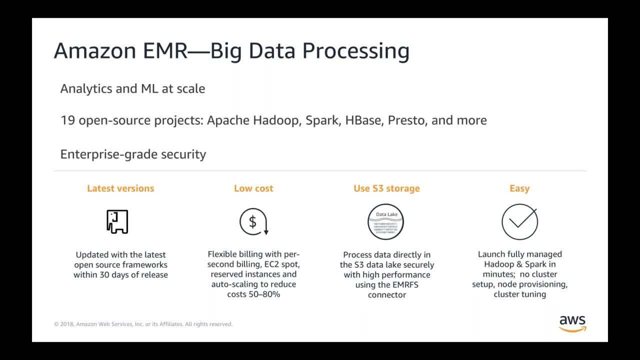 automatically replacing poorly performing instances. Amazon EMR automatically configures EC2 firewall settings that control network access to instances and you can launch clusters in an Amazon virtual private cloud, a logically isolated network you define For objects stored in Amazon S3, you can use Amazon S3 server side. 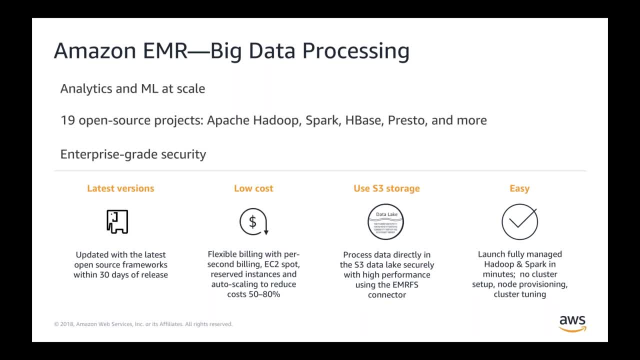 encryption or Amazon S3 client side, EMR, FS. with key management service or custom managed keys, You have complete control over your cluster. You have root access to every instance. You can easily install additional application and you can customize every cluster. with bootstrap action. You can also 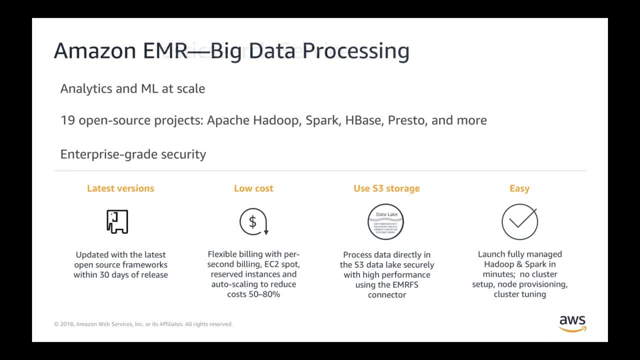 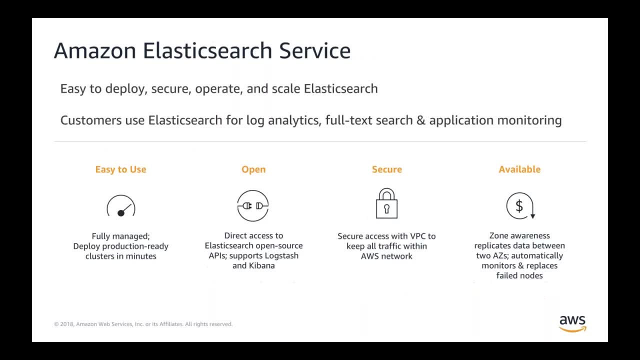 launch Amazon EMR clusters with custom Linux AMIs, which reduces your bootstrap times. The next service on the analytics space is the elastic search service. The last Amazon elastic search service makes it easy to deploy, secure, operate and scale elastic search for log analytics. 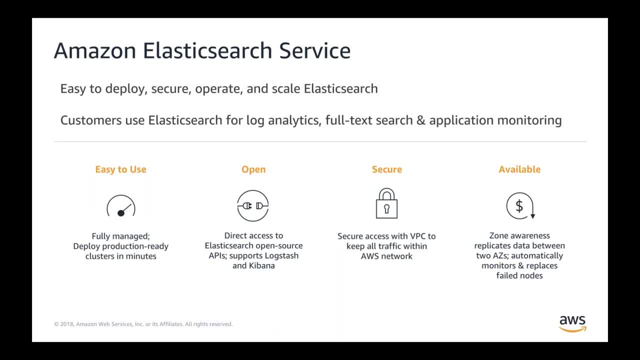 full text search, application monitoring and more. Amazon elastic search service is a fully managed service that delivers elastic search, easy to use APIs and real-time analytic capabilities, alongside the availability, scalability and security that production workloads require, The service offers built-in integrations. 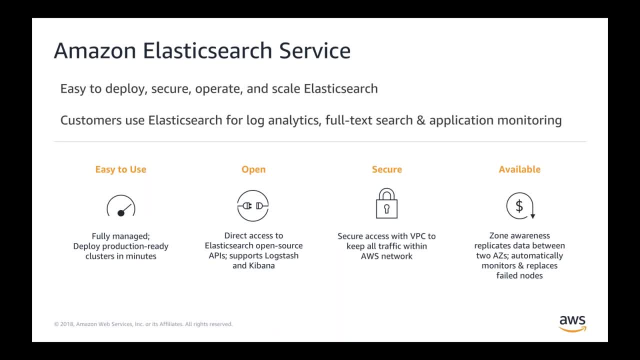 with Kibana, Logstash and AWS services, including VPCs, Kinesis, Firehose, Lambdas and CloudWatch, so that you can go from raw data to actionable insights quickly and securely. It's easy to get started: with Amazon elastic search service, You can. 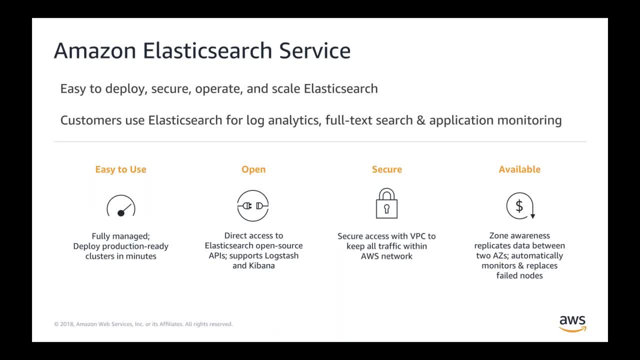 set up or configure your Amazon elastic search service domain in minutes from AWS management console. Amazon elastic search service provisions all the resources for your domain and launches it. You can securely set up and configure your Amazon elastic search domain in minutes from the AWS management console With Amazon elastic. 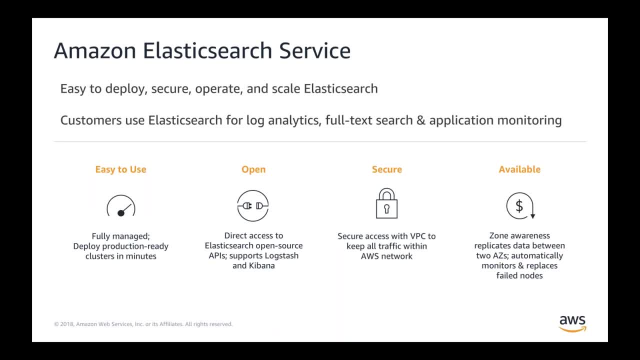 search service. you get direct access to elastic search open source API, so the code and applications you're already using with your existing elastic search environments work seamlessly. The four services that we spoke about now- Amazon, Athena, Redshift, EMR and elastic search- are: 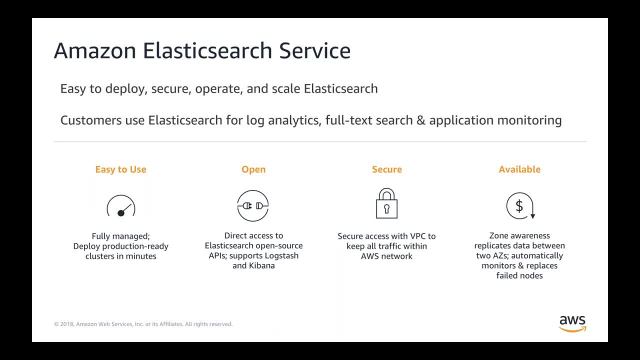 your absolute best access layers from your data lake. Your access layers can be anything. It can even be an Aurora PostgreSQL database, depending on what your end users require. For them to take actionable insights, they need a visual analytics tool, And that's where I would like to. 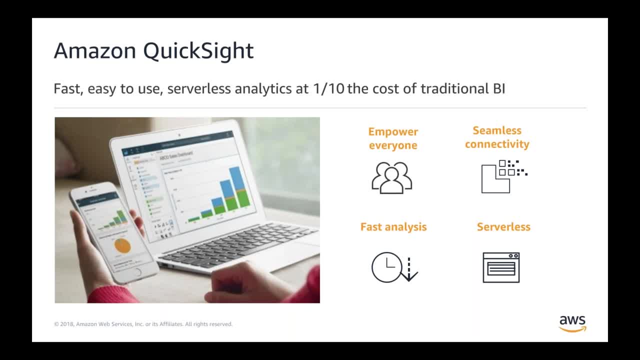 introduce Amazon QuickSight, a fast, cloud-powered business analytics service that makes it easy to build visualizations, perform ad-hoc analysis and quickly get business insights from your data. Using our cloud-based service, you can easily connect your data, perform advanced 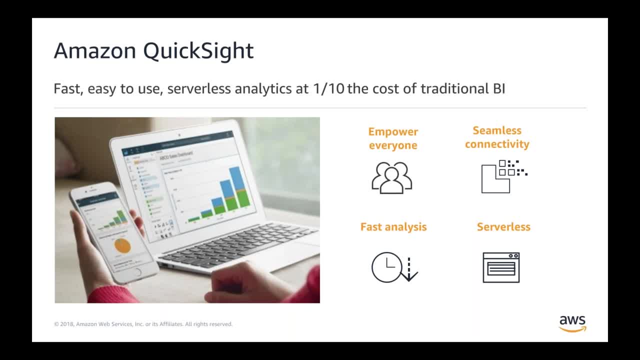 analysis and create stunning visualizations and rich dashboards that can be accessed from any browser or mobile device. QuickSight enables self-service, decentralized analytics in your organization better than any other system out there. As a business analyst, you can take an analysis from a concept. 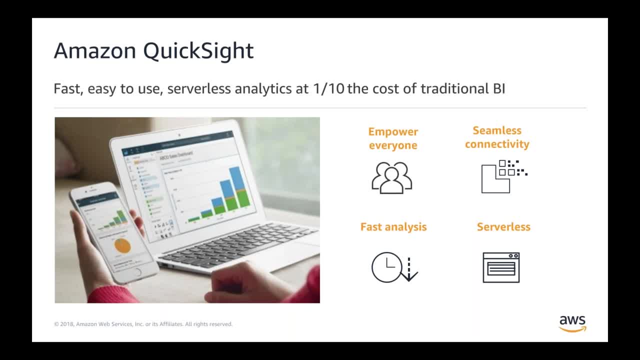 to reality without depending on data engineers. You can create and prepare data sets, build your analysis and share collaboration with little or no intervention from IT or data engineers. Connecting to a data source, especially AWS data sources, doesn't involve back-end coding or complex setup. You simply 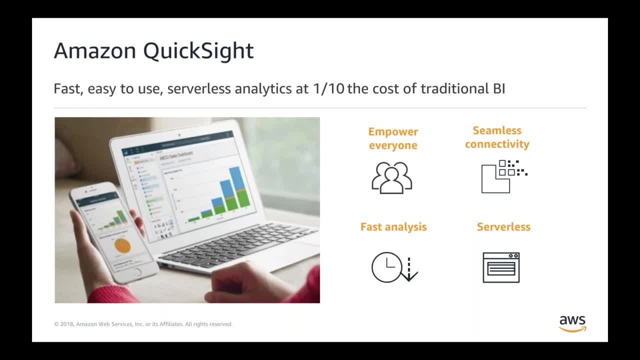 click on the data source and enter your credentials and QuickSight will auto discover tables that you can select from taking out the guesswork, from selecting the right table to create your data sets. Then there is scheduled refresh. If you set up your data set to refresh every day, every. 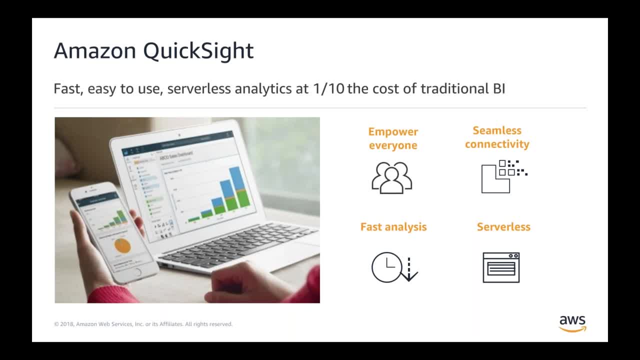 week. then you're assured of the latest data when you're looking at your analysis. Fast interactions with your charts and graphs. The charts and graphs built on Spive's data are really responsible, Responsive. You can zoom in, zoom out, drill. 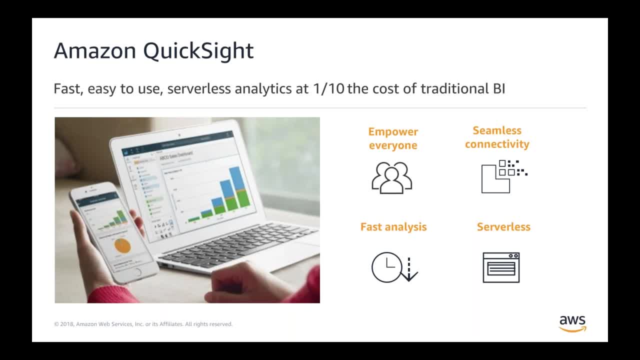 through add filters on the fly with little to no time delay. With QuickSight, you can do anything. It's completely serverless. Not only do you need- do you not need to install anything or deploy for QuickSight, but in 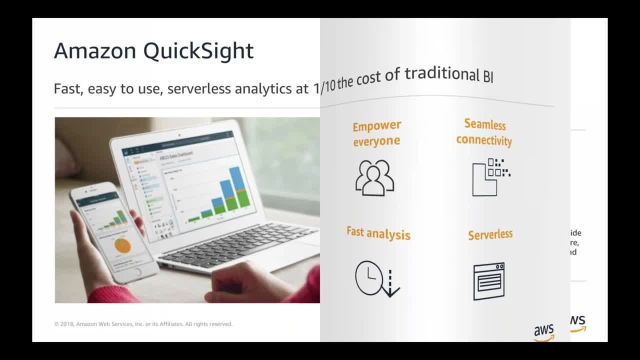 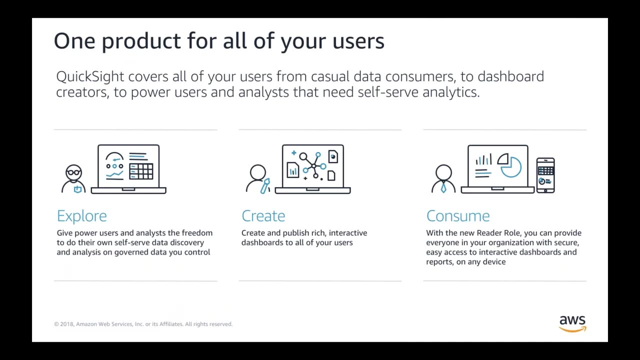 combination with S3 and Athena, you can have an end-to-end analytic solution without ever starting or managing a server. QuickSight is one product for all your users. We give proper users and analysts the freedom to do their own self-serve data discovery and 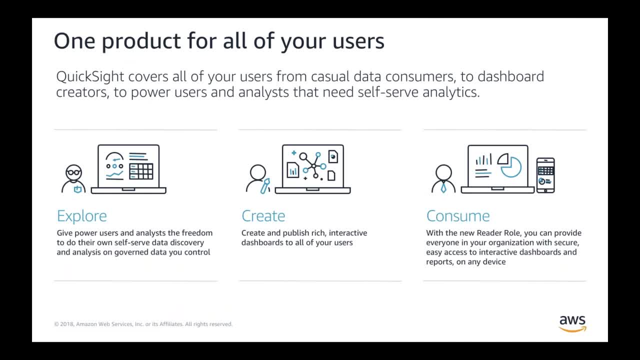 analysis on governed data. you control, Create and publish rich interactive dashboards to all of your other users And, with the new reader role, which I'm going to talk about in a bit, you can provide everyone in your organization with secure, easy access to interactive. 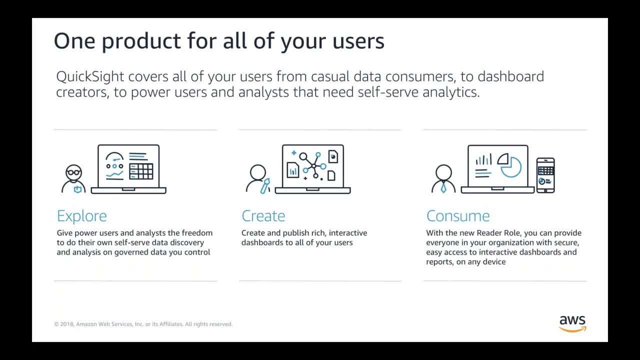 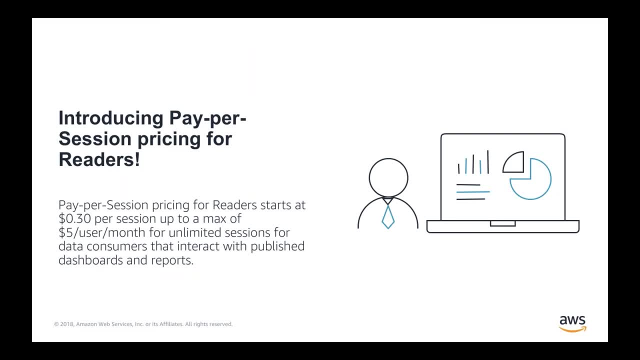 dashboards and reports on any device, So with readers. we also introduced pay per session pricing, So you only pay for the session at 30 cents per session, up to a maximum of $5 per user per month for unlimited sessions for data consumers. that. 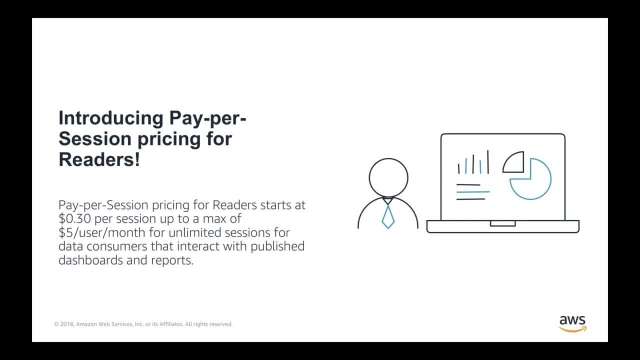 interact with published dashboards and reports. Think of this as your floor manager, who wants to look at a report before he gets into the stand-up in the morning. He doesn't have to be a power user for QuickSight. He can be termed as. 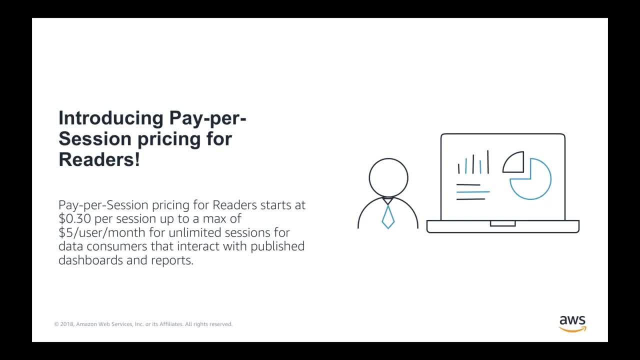 a reader and he only pays per session pricing for the reader. So he would only pay 30 cents to actually look at a report before he enters into the stand-up. If he looks at the report multiple times in the day, then he will only. 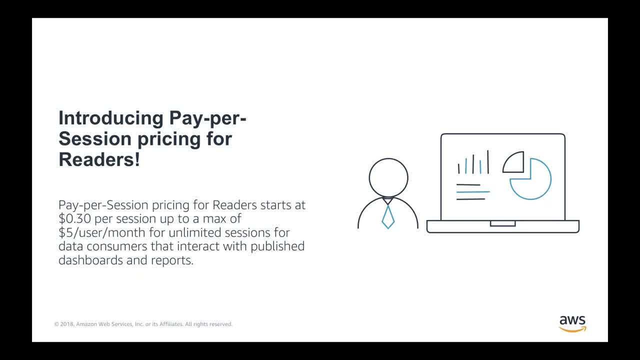 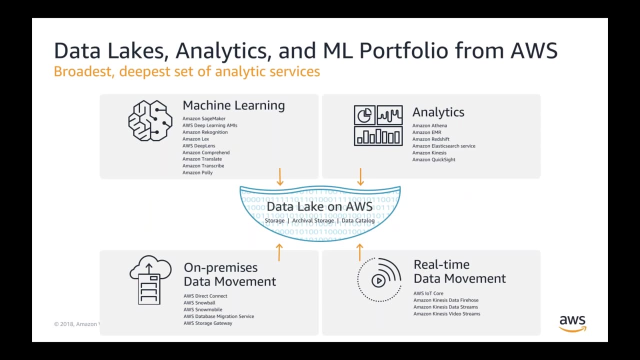 pay 30 cents for every session to a maximum of $5 per user per month. That is really being cost effective and that is really giving the power of analytics to your end users. The next step in data analysis from Data Lake is machine learning. 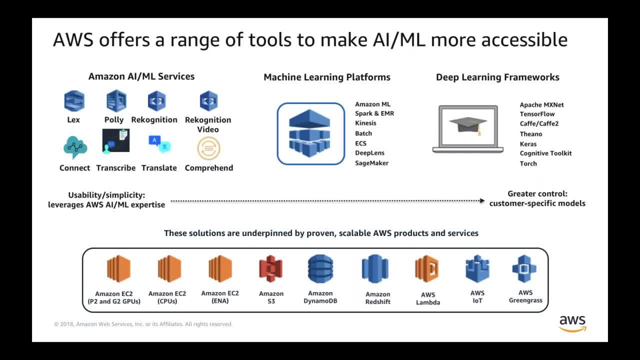 AWS offers a range of tools to make AI ML more accessible. It provides you Lex Poly Recognition for facial recognition. Connect, the Amazon Connect service Transcribe, which allows you to transcribe your text, Translate and Comprehend, which is the natural language processing. 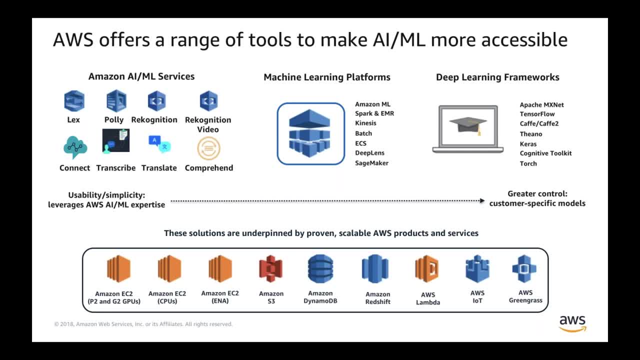 engine And it also supports the machine learning platform, which supports Amazon, ML, Spark and EMR, Kinesis, Batch, Elastic Container Service, DeepLens and SageMaker. It also supports deep learning frameworks like Apache, MXNet, TensorFlow, Cafe, Tiano, Torch. 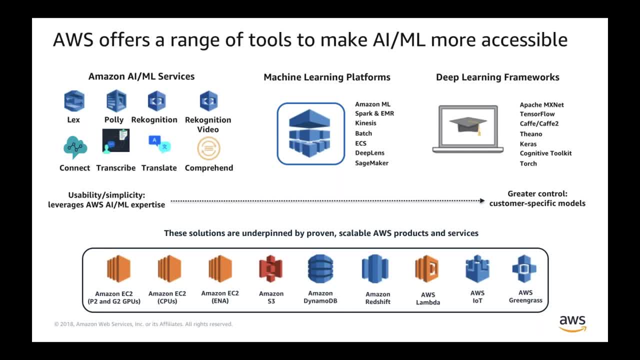 and, if you look at it, the usability and simplicity are on the left hand side, where you use the AI services that we provide and you get greater control and customer specific models when you use Apache, MXNet or TensorFlow to develop your own models. These solutions are underpinned by proven 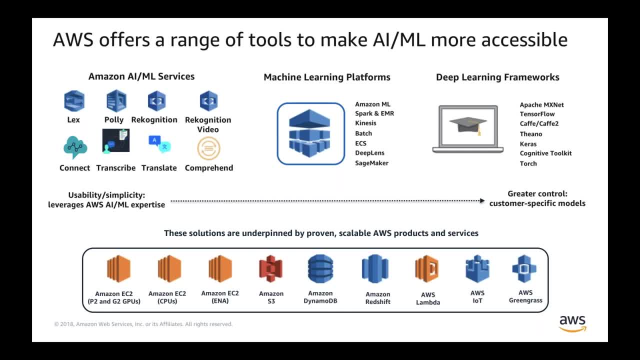 scalable AWS products and services like EC2s with P2 and G2 GPUs, Amazon EC2 instances with CPUs, Amazon EC2s with elastic network adapters, Amazon S3- scalable, highly durable storage service. DynamoDB, highly scalable, highly available NoSQL database, petabyte. 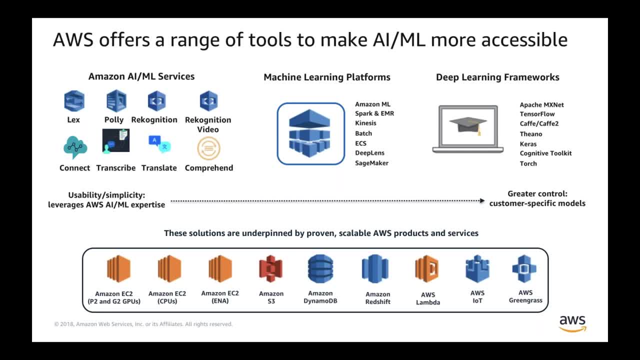 scale data warehouse, which is Redshift. Lambda, which is a serverless technology for running your event driven functions. AWS IoT for interacting with your internet of things. So these services in total give you a range of tools to make AI ML more accessible: Amazon SageMaker. 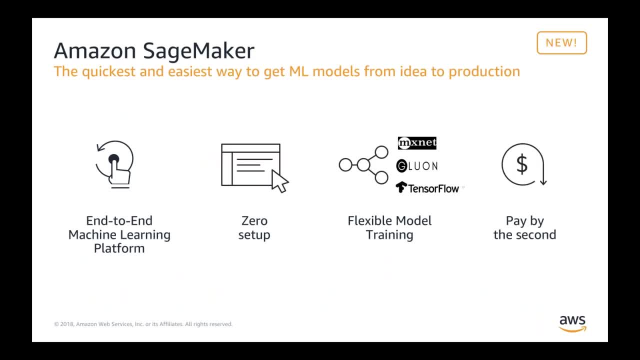 removes the complexity and holds back developer success. with each of these three steps, SageMaker includes models that can be used together or independently to build, train and deploy your machine learning models. Amazon SageMaker is fully managed platform that enables developers and data scientists to quickly 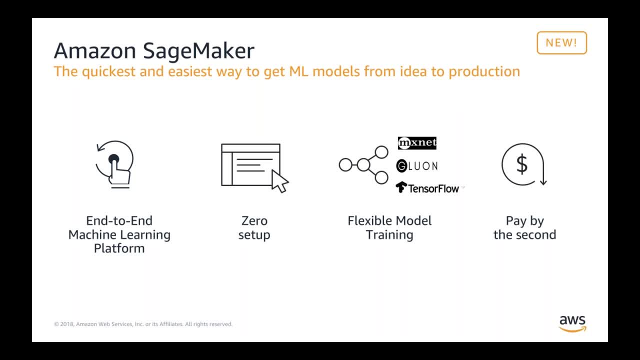 and easily build, train and deploy machine learning models at any scale. Amazon SageMaker removes all the barriers that typically slow down developers who want to use machine learning. SageMaker significantly reduces the amount of time needed to train, tune and deploy machine learning models. 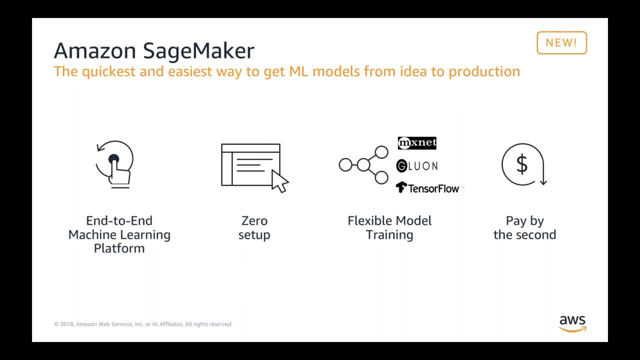 manages and automates all the sophisticated training and tuning techniques so you can get models into production quickly. Amazon SageMaker supports all machine algorithms and frameworks so you can use the technology you are already familiar with. Apache, MXNet and TensorFlow are pre-installed. 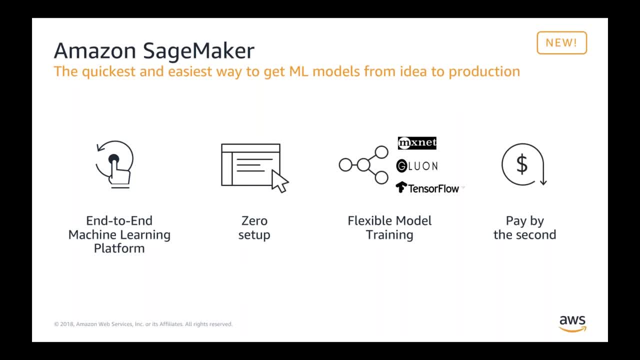 SageMaker offers a range of built-in high performance machine learning algorithms. If you want to train with an alternative algorithm, you can bring in your own Docker containers as well. SageMaker lets you begin training your model with a single click in the console or with a single API call. 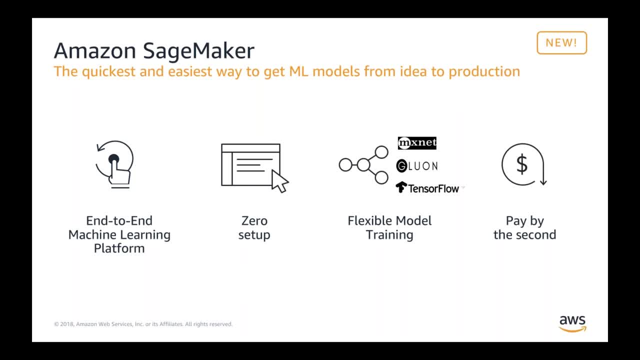 When the training is complete and you are ready to deploy your model, you can launch it with a single click in the Amazon SageMaker control. It integrates with your existing workflows. It allows you to integrate machine learning models into your application by providing an HTTPS endpoint. 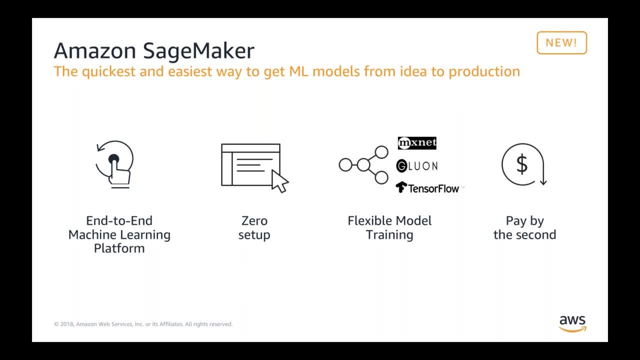 that can be called from any application, Which basically means your application can call an API to get real-time predictions from SageMaker. SageMaker is pre-configured with the latest version of TensorFlow and Apache MXNet with CUDA 9 library. support for maximum performance with NVIDIA GPUs. 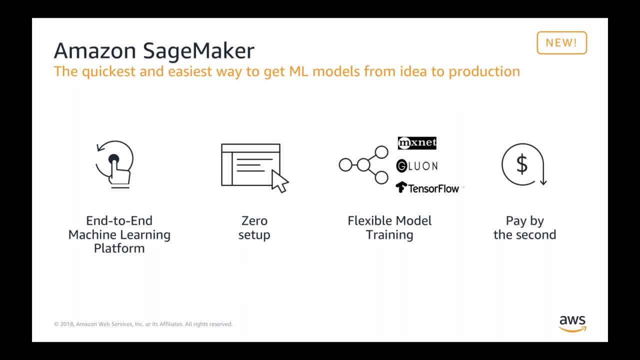 With Amazon SageMaker P3 instances running NVIDIA Volta V100 GPUs. Amazon SageMaker lets you train deep learning models with unparalleled speed. Recently, we also released a blog post on how you can use a SageMaker with EMR for you to use Spark ML models. 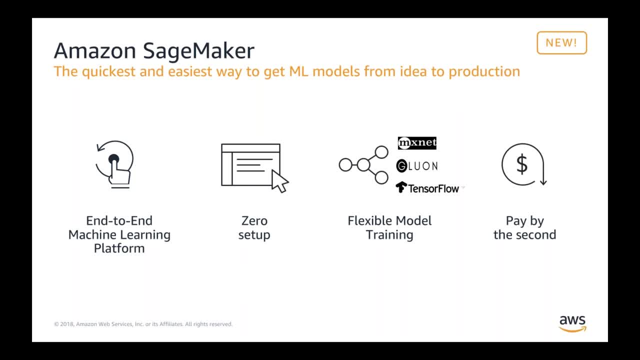 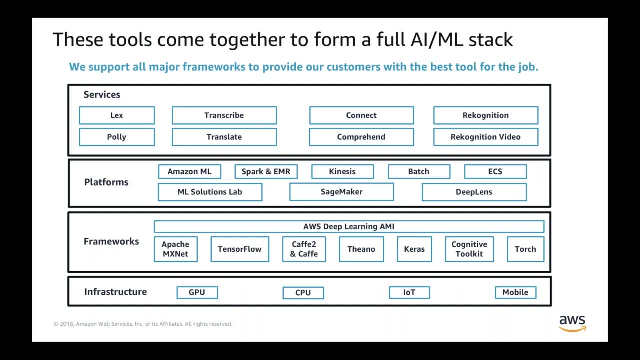 if you want to use Spark ML models. Again, SageMaker is pay-per-second, so you only use it when you are actually consuming the models or training the models. You don't pay for when you are not actually running the models. So 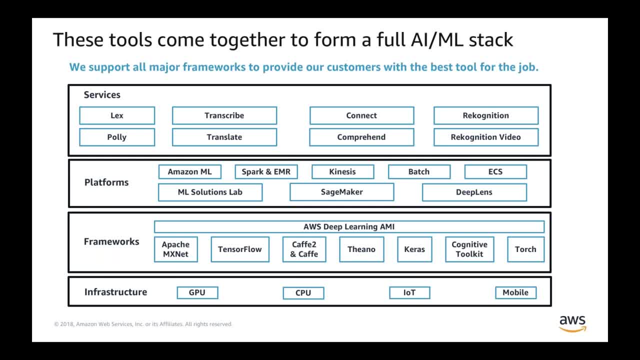 the big picture. these tools all come together to form the full AI ML stack. So we have lot of services on the top box which are fully managed by AWS. There are platform services that gives you flexibility. platform and frameworks that give you flexibility. 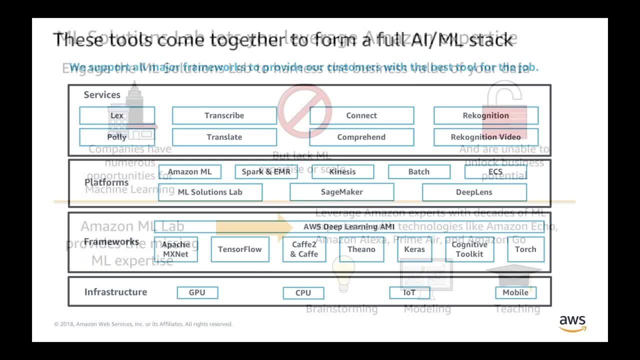 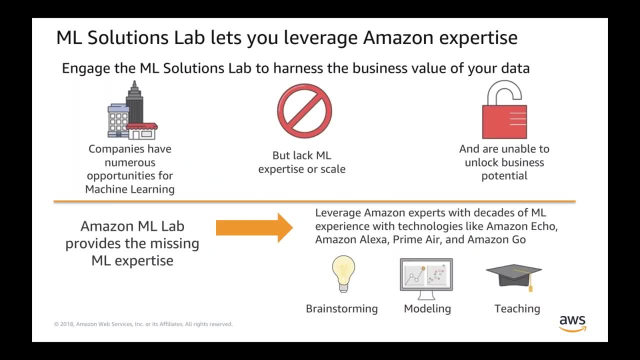 to build your own models and infrastructure to run all these at scale. The ML Solution Lab lets you leverage Amazon expertise and you can use numerous opportunities for machine learning, but you lack the ML expertise or scale and are unable to unlock business potential. The Amazon ML Lab provides. 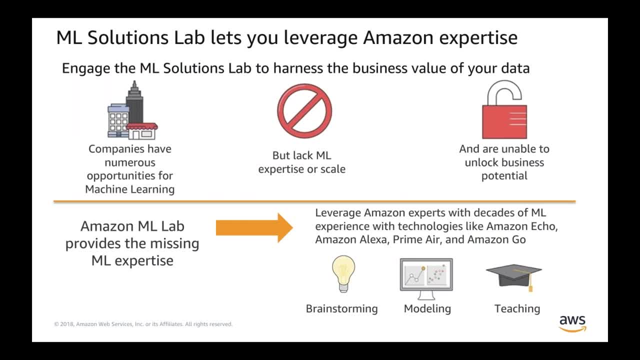 the missing ML expertise. Leverage Amazon experts with decades of ML experience with technologies like Amazon Echo, Alexa Primer and Amazon Go. The Amazon AI Lab is available to consumers with AWS Business Support or AWS Enterprise Support. Please reach out to the Amazon account team if you are. 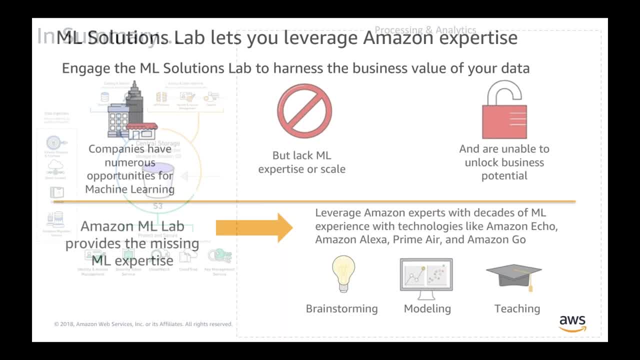 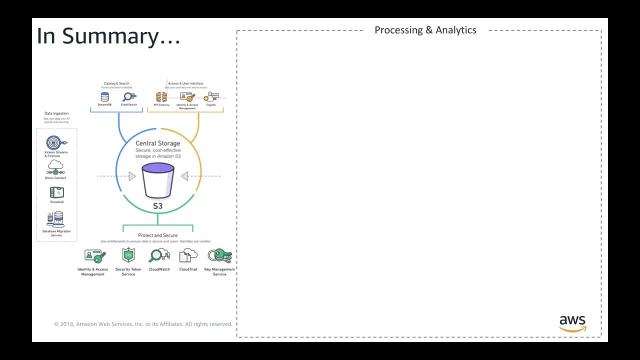 interested in doing a ML Solutions Lab with AWS. So, in summary, I have data that is getting ingested from various sources. So I have data ingestion happening via Kinesis Streams, via Direct Connect, Snowball, Snowmobile Database Migration. 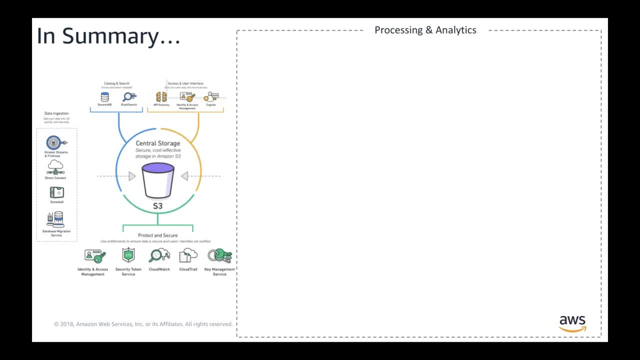 Service into S3.. I use DynamoDB and Elasticsearch to catalog and search the data. I use the API Gateway to give access and user interface for the data stored in the data lake. We also use IAM Security, Token Service, CloudWatch, CloudTrial and Key Management. 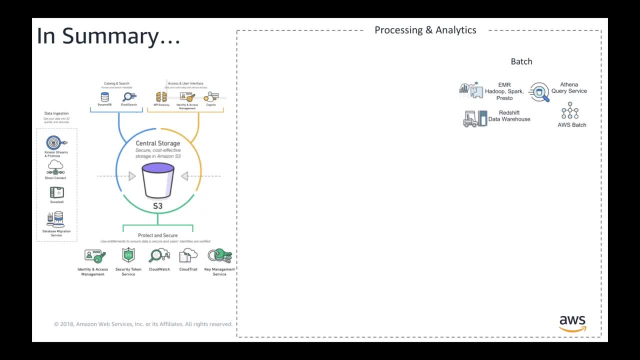 Service to protect and secure the data. For processing and analytics we can use batch processing like EMR, Athena Redshift Data Warehouse or AWS Batch. We can use traditional RDBMS, DynamoDB or Aurora relational databases. This all depends on what your end user needs. 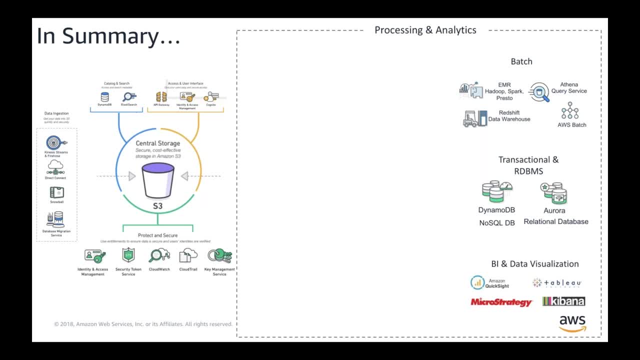 You cannot choose a service until you know your use case. So you understand your business use case and come back and say: this is a batch use case, this is a transactional use case, transactional RDBMS use case or a NoSQL use case. 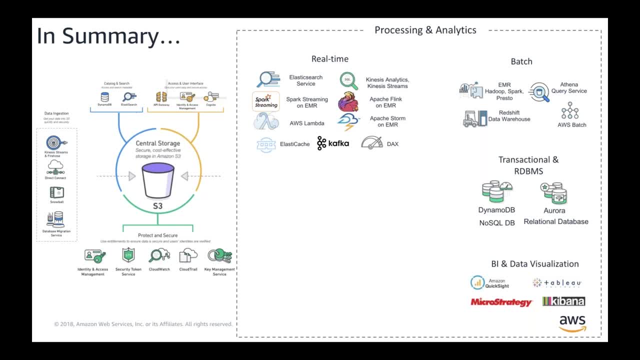 You use BI and data visualization. QuickSight is available. You can also use Tableau, MicroStrategy, Kibana, QlikView to do your BI and data visualization. You also have real time services like Elastic Search Service, Kinesis Analytics. 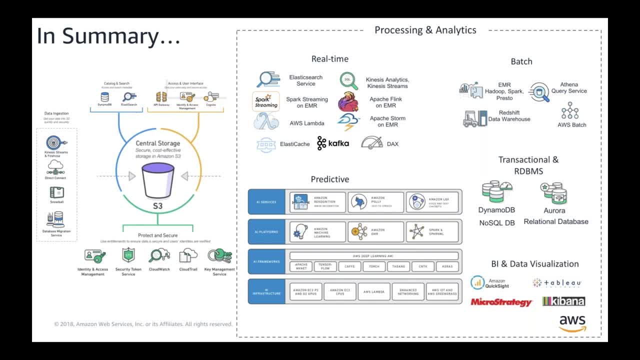 Apache Flink running on EMR, Spark, streaming on EMR, Elastic Cache, Kafka and DAX, which gives you real time access to the data. And then you have got the predictive services, which allows you to do AI services like LEX recognition. 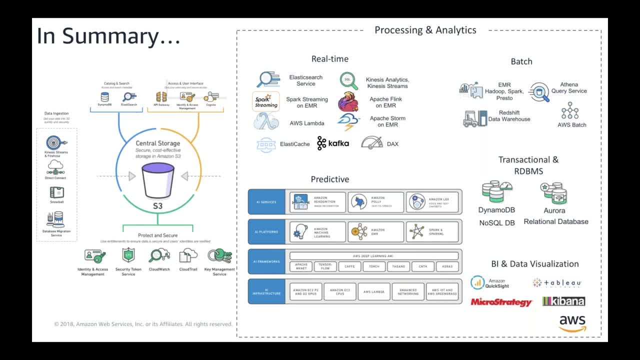 AI platforms like Amazon EMR, Spark, Spark ML, Amazon Machine Learning, AI frameworks for AWS, deep learning, AMEs, all the AI infrastructure on EC2, P2s, G2s and GPUs. For all this to work, you need a central storage. 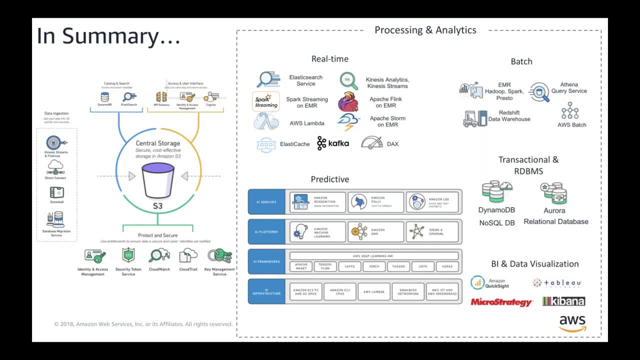 a secure, cost effective storage, which is Amazon S3.. So you start your data lake project on AWS by utilizing Amazon S3 as your central storage to store all your data. bring data into S3, use Glue to further transform the data, to enhance the data, enrich the data. 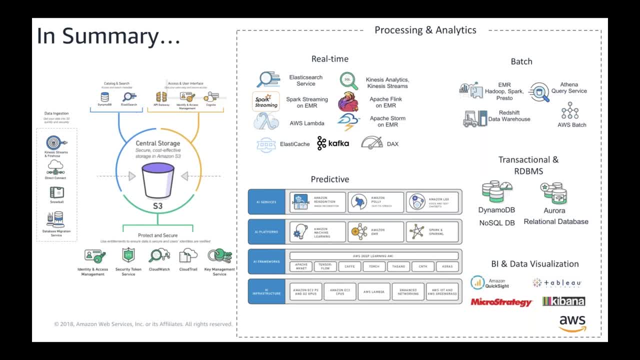 and load it into the data lake, and also load it into other services like Redshift, or use it on Elastic Search Service And then create BI and visualization on it, or use predictive analytics on top of it. Now that you've attended the webinar and are interested in learning, 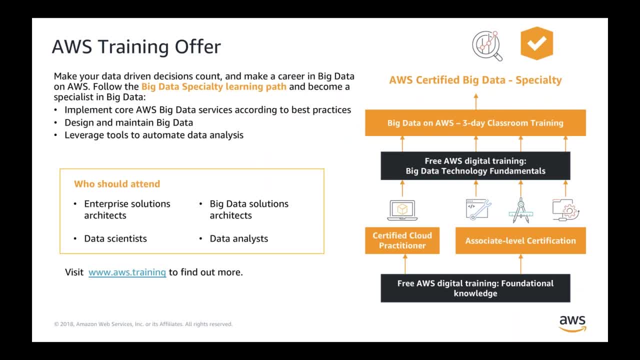 more. what do you need to do next? Visit the AWS training portal. sign up for our online digital training. Here you can explore a number of free courses relating to big data, machine learning and the internet of things. We offer a three day big data. 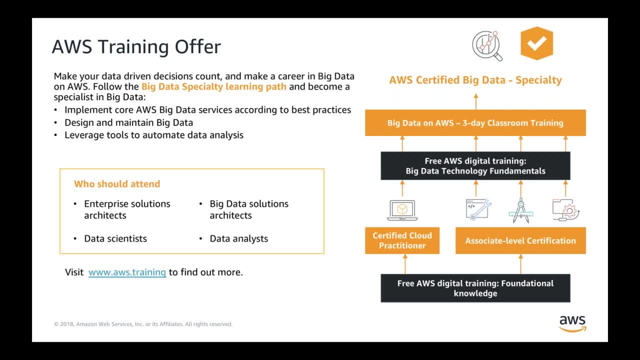 on AWS specialty course where you will learn how to work with Amazon EMR, Amazon Redshift, Amazon Kinesis, Amazon Athena and Amazon and the rest of the AWS big data platform to process data and create big data environments. We also offer a big data. 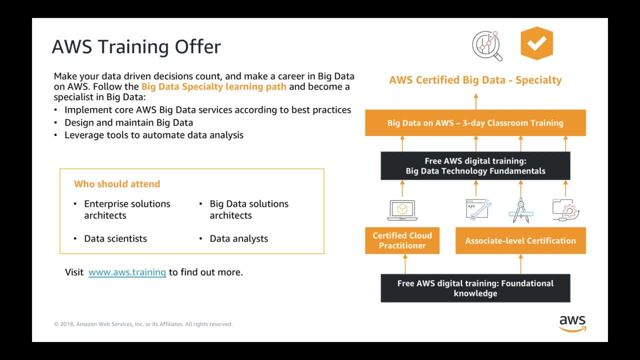 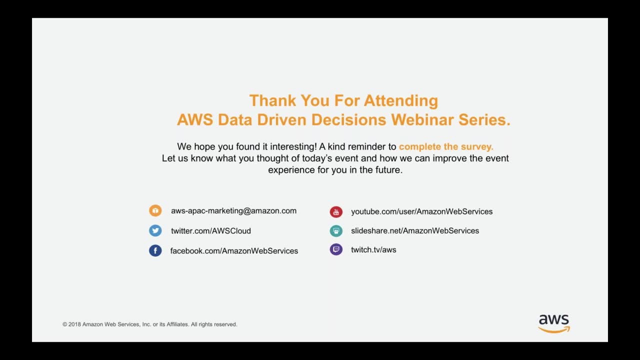 specialty certification, which is integral to anyone working in this area. Don't forget that you need to obtain a foundational cloud practitioner certification or an associate level certification before you can qualify to sit the specialty certification. Visit the training website at awstraining to know more and get started today.